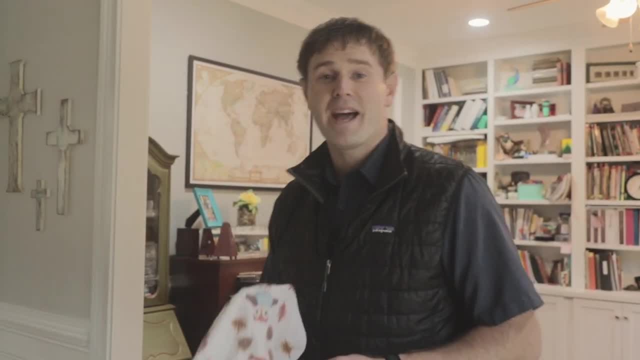 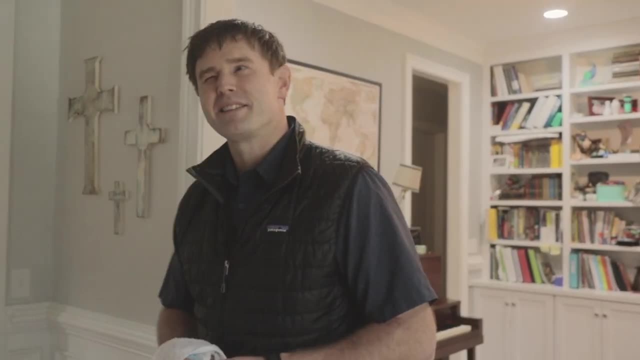 All right, So let's get started. What is your name? My name is Matt Threadgill. And what is your specialty? I'm a pediatrician. And how many years have you been practicing? I've been practicing 10 years in private practice. All right, And where did you go to undergrad? Went to undergrad. 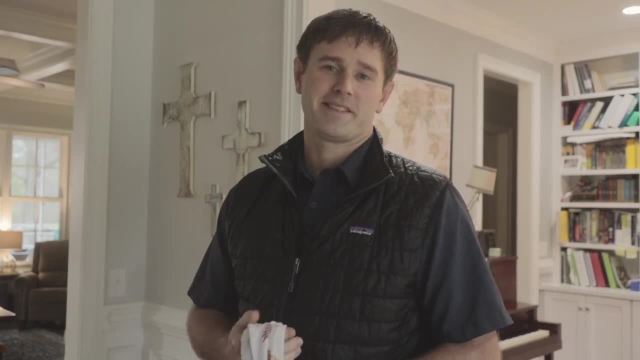 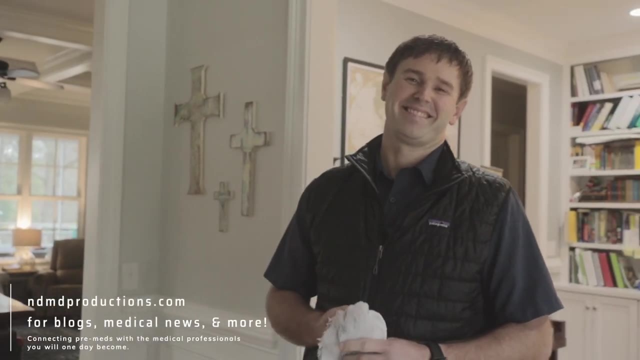 at the University of Georgia in Athens And medical school- Medical school at the Medical College of Georgia, Nice. I'm familiar with that a bit. Yeah, I hope so. Did you take any gap years before going to medical school? I did not. I went straight from college to medical school. 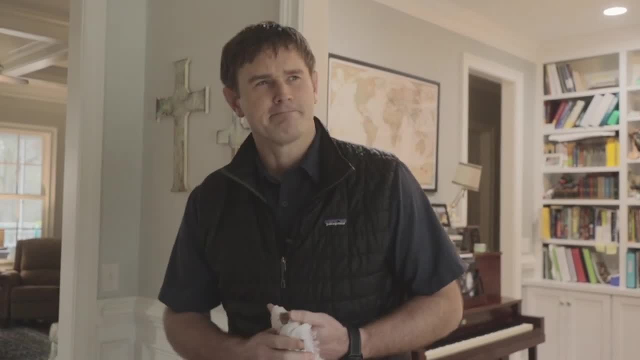 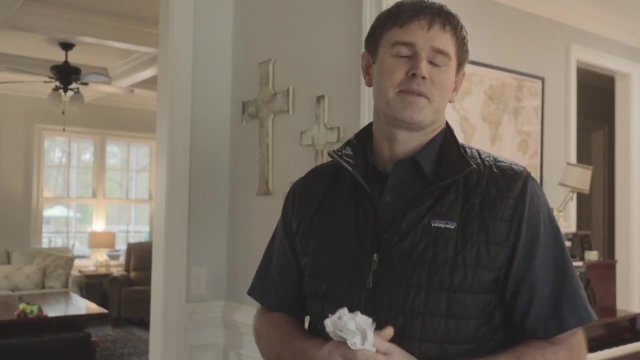 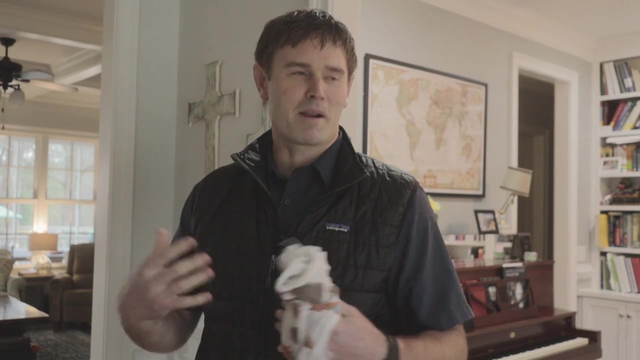 What was your favorite part of medical school? My favorite part of medical school would have to be medical school. It would have to have been the community of brothers, the brotherhood we had amongst each other. in my class That's probably the thing that sticks out the most. Very well said What. 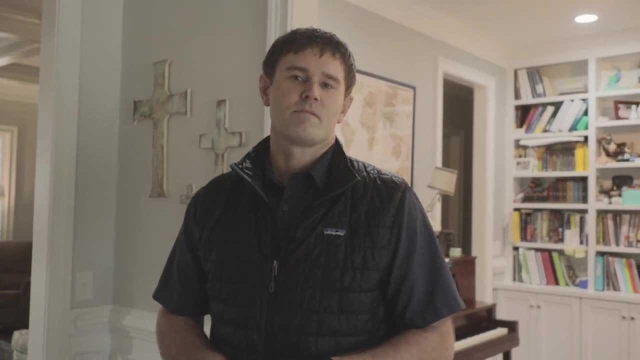 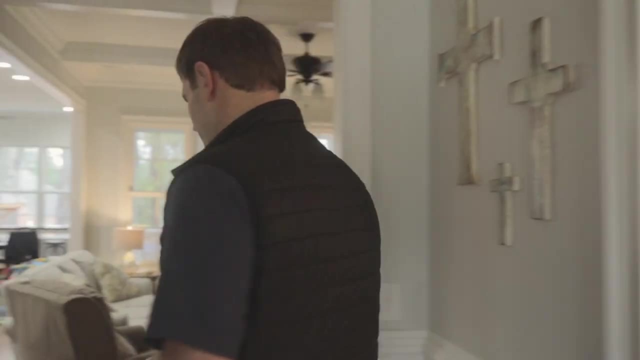 specialty did you think you were going to go into on your first day of med school? Honestly, I thought family medicine was probably what was going to be the best for me. Let's wander around here in the kitchen, Sure, But I didn't know. 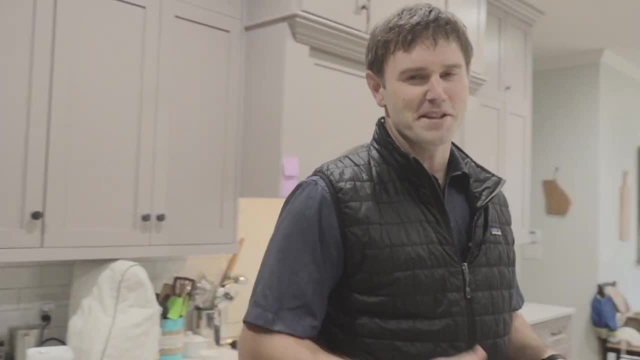 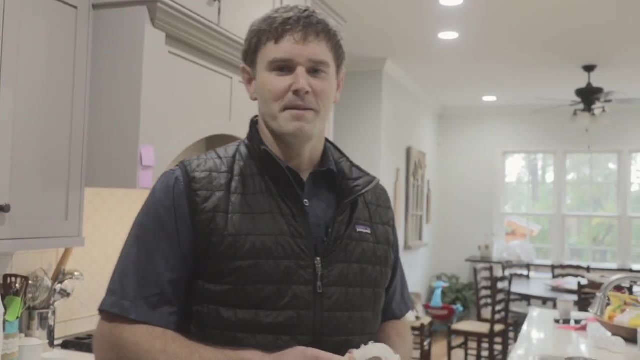 I didn't know much about it, other than having hung out with my family physician, for you know a little bit here and there before I went to medical school, So didn't have a good clue about what that looked like. All right, Well, what changed your mind about that specialty family? 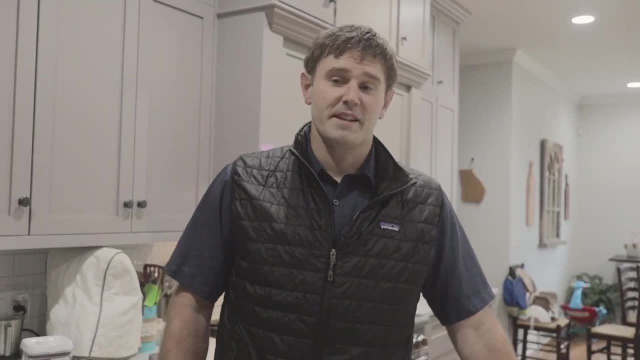 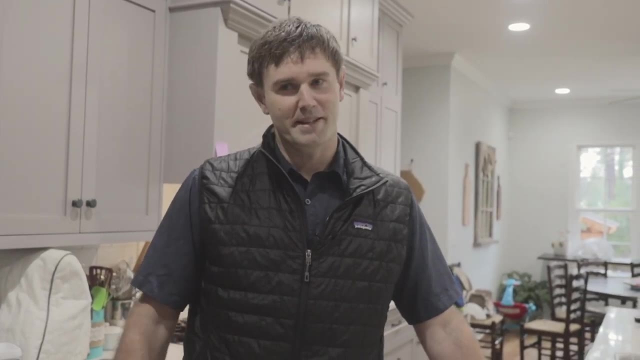 medicine. Well, I actually loved family medicine. I did a family medicine rotation at a very rural site in Edgefield County, just up the road here, And they were just this amazing family medicine staff and had me convinced that I was going to go into medical school And I was like, oh my God. 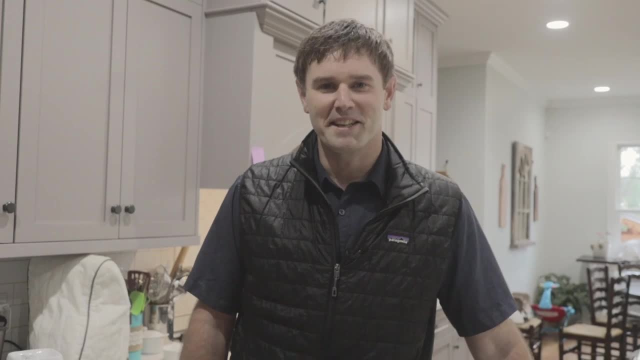 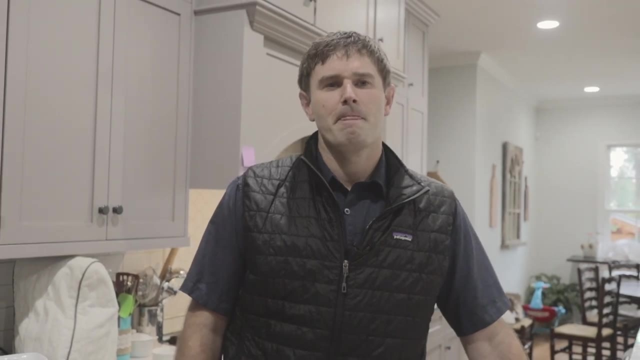 I'm going to go into family medicine. But that all changed late in my third year of medical school when I rotated through pediatrics. All right, Were there any specialties? you immediately said not for me, Absolutely not. You know, I never, really, I never really had that experience. 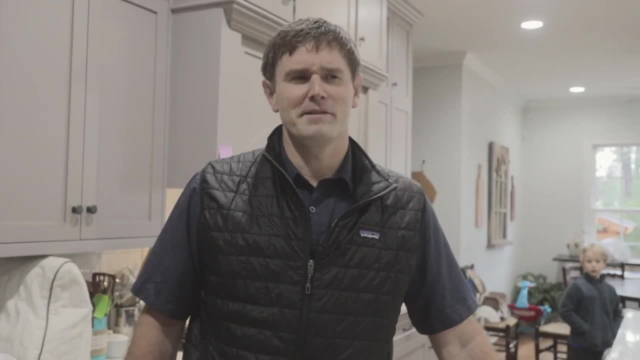 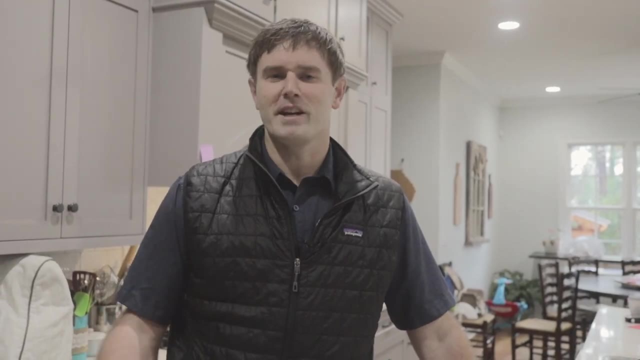 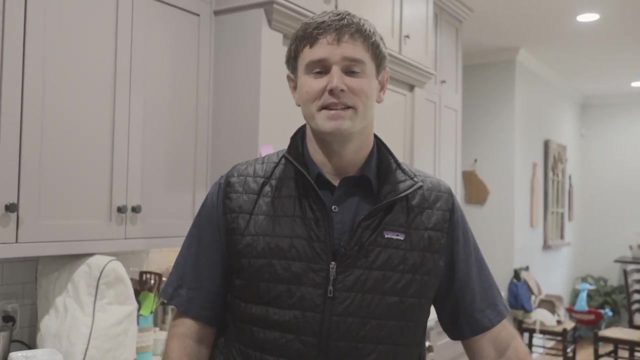 in medical school. You know I really enjoyed every single rotation, even psychiatry. I mean there was beauty in interviewing and learning about people's stories and just somehow those stories just get broken. And how can we enter into that brokenness and help people? through even mental illness. That's awesome. So how long does your training as a pediatrician take after med school? So after medical school? if you are, like me, a general pediatrician, then there's three years of residency after medical school. Okay, And I know I guess you 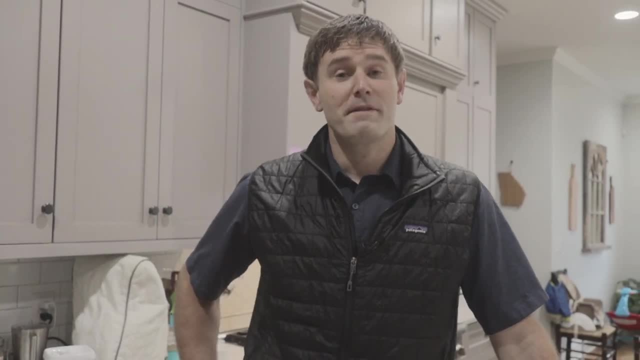 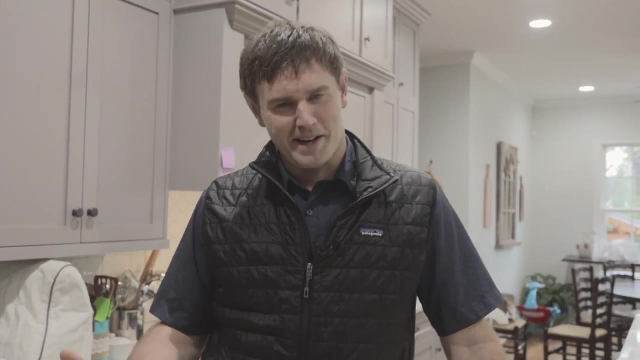 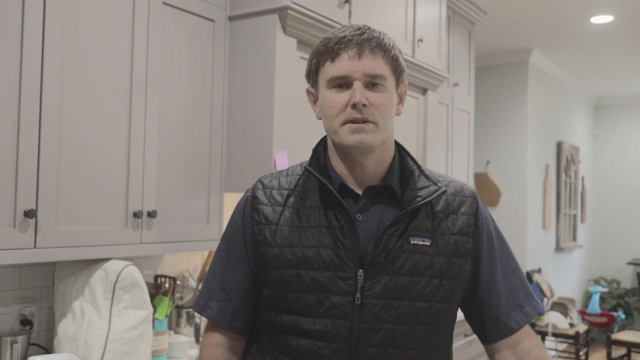 answered this question earlier, but are you in academics or private practice? I'm in private practice, And what do you like about private practice over academics? Well, I should say we're mostly private practice. We do have medical students that do rotate through our clinic And we occasionally have students shadowing who are thinking about 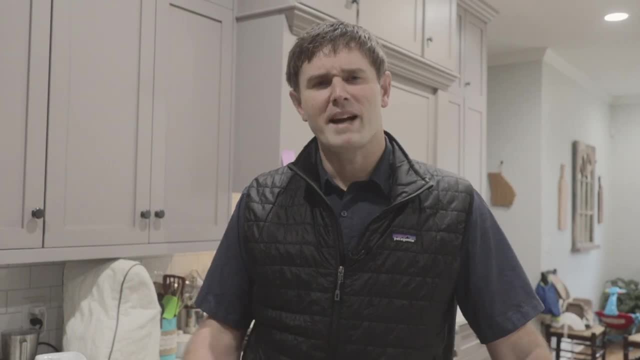 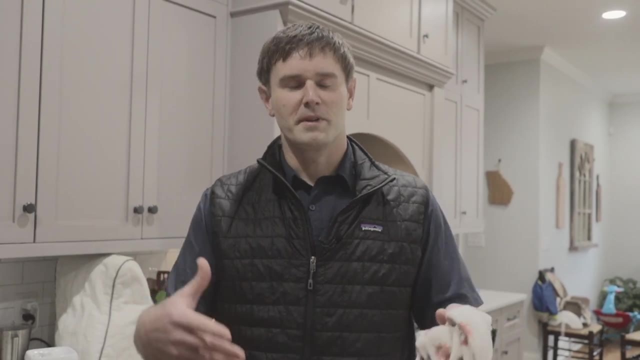 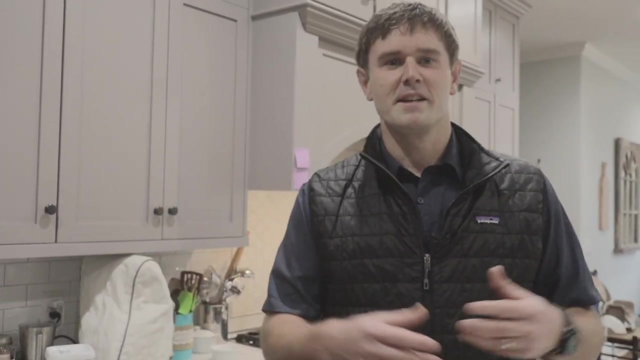 medical school coming through the clinic. But private practice in general to me is just that there's a lot of relationship, focus on relationships with families, that you know I'm not juggling a lot of other things besides my patients. That's awesome And I guess we'll try to keep it positive. but I do want to ask: are there any cons that you think? 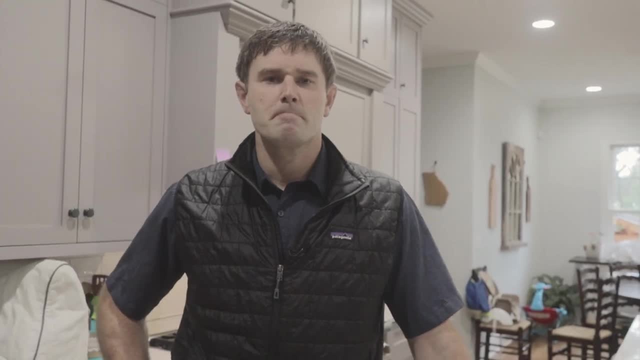 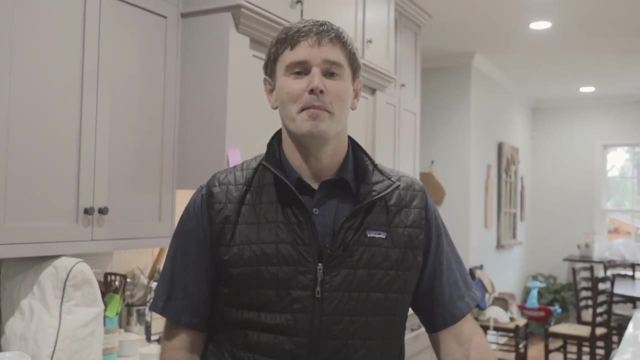 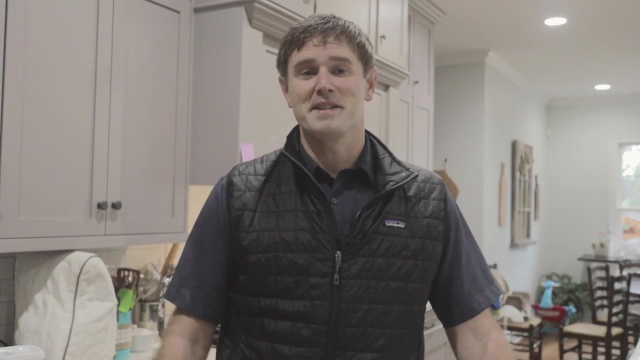 about private practice over working in a hospital, or at least major differences. You know, I think every time we have a student come through I'm always just delighted to be a part of just their formation and speaking into their life, even as it pertains to medical education. 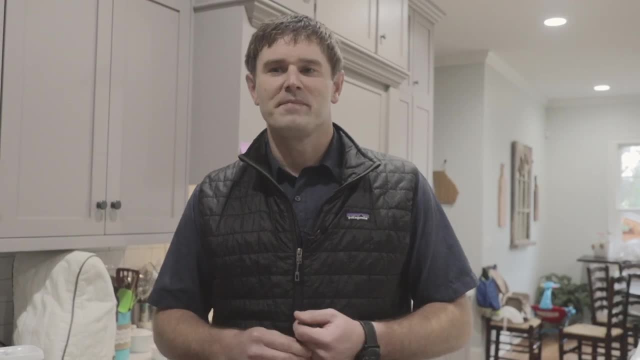 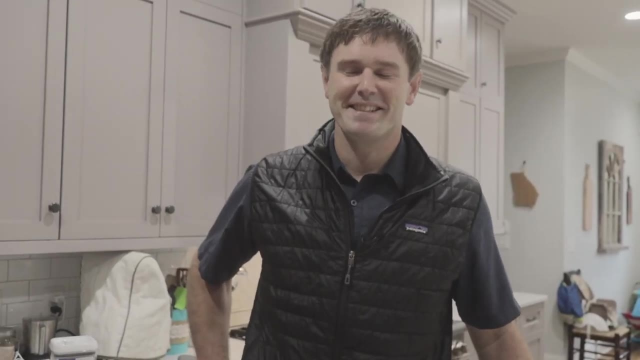 So, you know, having that as much, um, you know that that that may be a con, um, you know, but again I'm, I'm made a conscious decision, uh, you know, to be in private practice and not in academics. Did you consider getting any other degrees like an MBA or an MPH? No, an MD was, uh, that was plenty Enough years. right, That was, that was plenty of years. What would you say is the most unique part of your specialty? 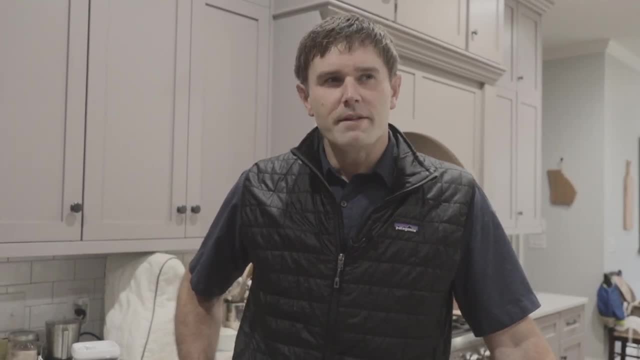 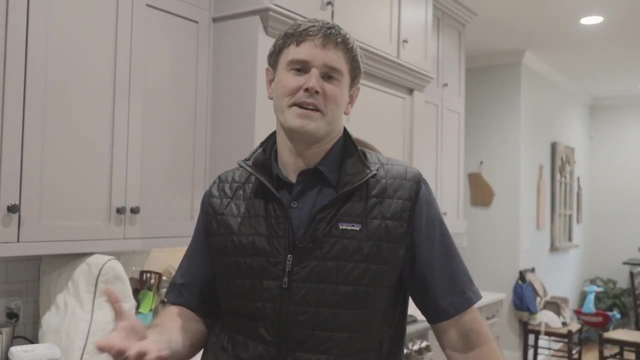 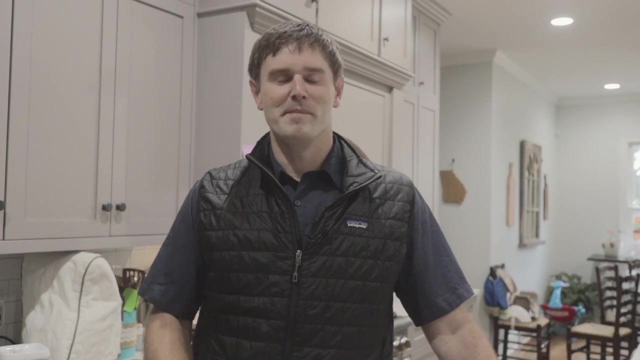 Um, I think the most unique thing about being a pediatrician um is going to be the long view, um, the long-term relationships that you have with people. You know we start with families from the very beginning, from pretty much in the delivery room, and walk with families through. 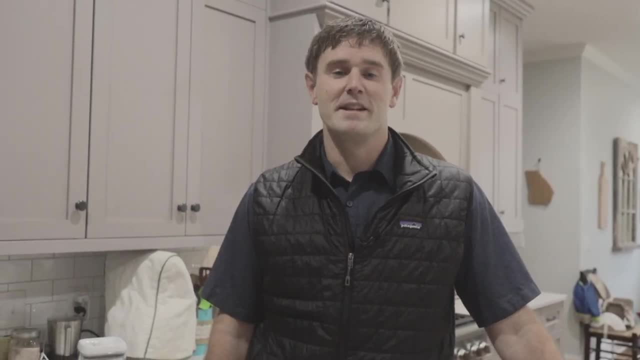 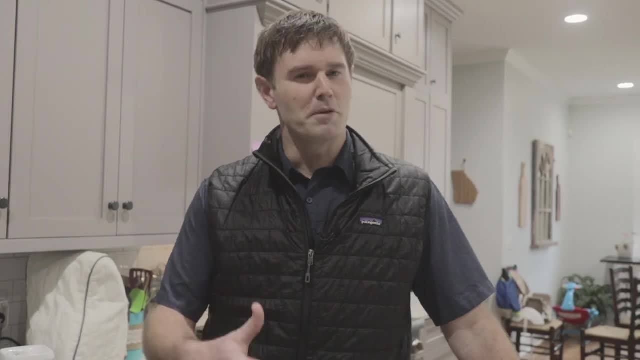 and so I think that's a very unique part of pediatrics- is being a part, a very close part of people's lives, Um and just these, uh, formative years, not only for the children, but for the parents too. 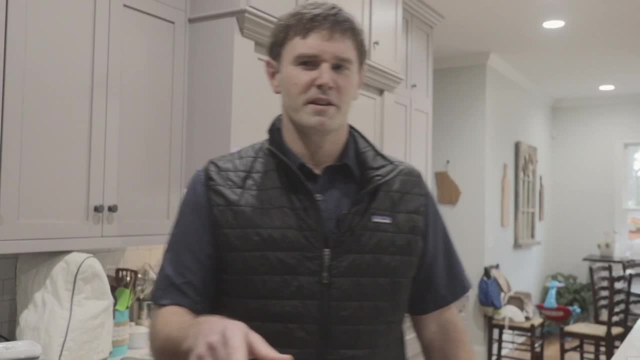 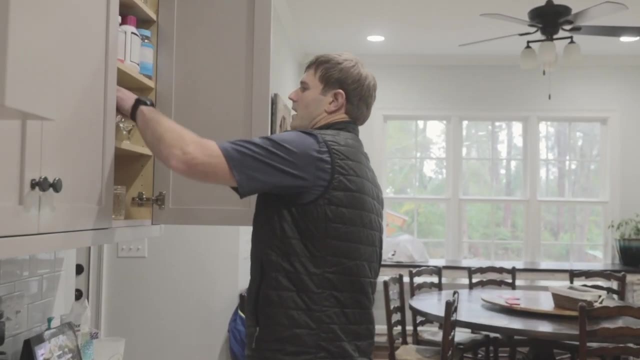 That's a great answer. So would you like something to drink? Um sure, Like some water, Just water. Okay, That'd be great. All right, Thank you, Yep. So why would somebody choose your specialty per se? Um, I think anybody who wants to choose pediatrics. you're really going to have to. 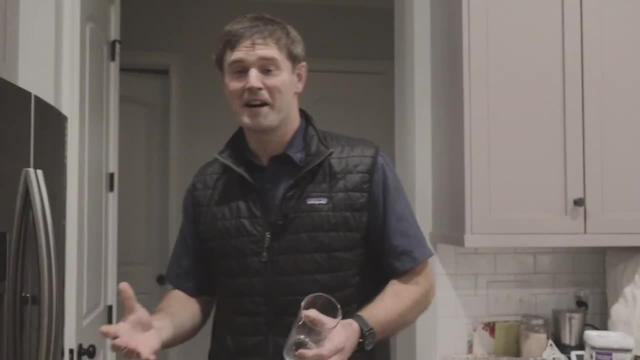 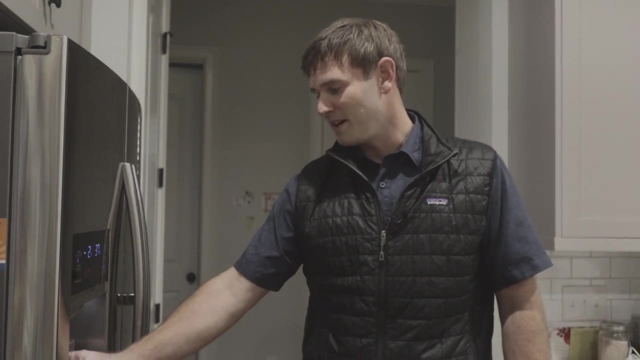 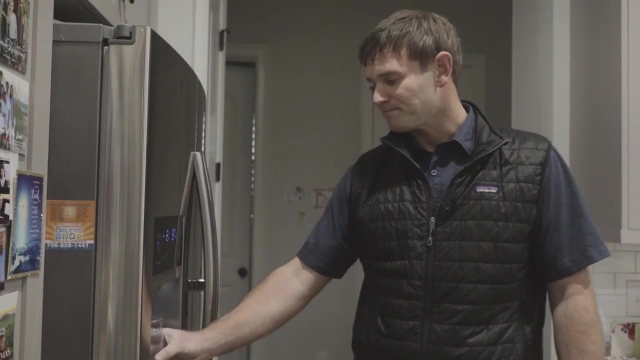 love preventative medicine for one. Um. so you know, pediatrics is preventative medicine. Um, you know we see a lot of checkups and um try to prepare people for what's coming next and protect children from, you know, disease and whatnot. Um so, um, I'm going to make a cup of coffee if that's okay. 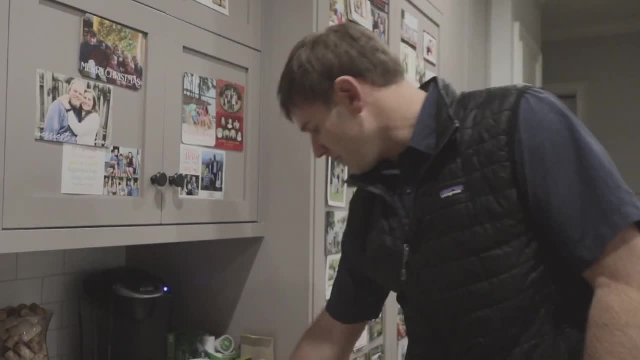 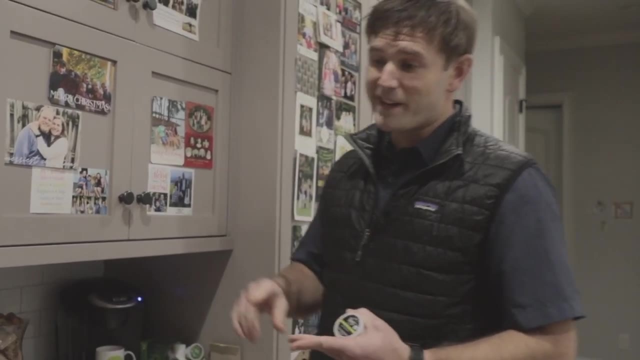 Of course, Um, the easy way through the Keurig, Um, so, uh, yeah, I think, I think that's what you got to love: Preventative medicine. You've got to love kids, I mean, um, so if screaming children doesn't, uh, if that puts. you off a lot, then you're probably not going to uh enjoy a day in the clinic, because sometimes our halls sound like, uh, like the London Tower. about the time of Henry VIII, I think. Um, occasionally there's a lot of screaming, Um, but uh, you know there's. 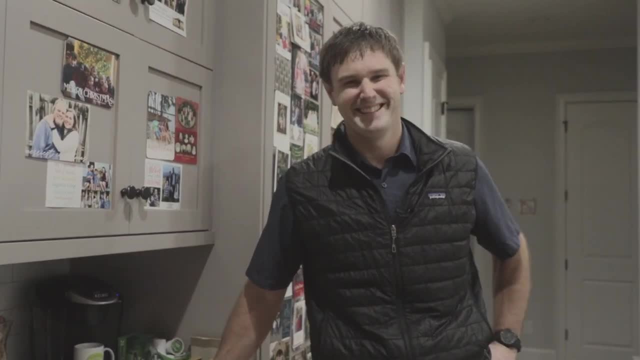 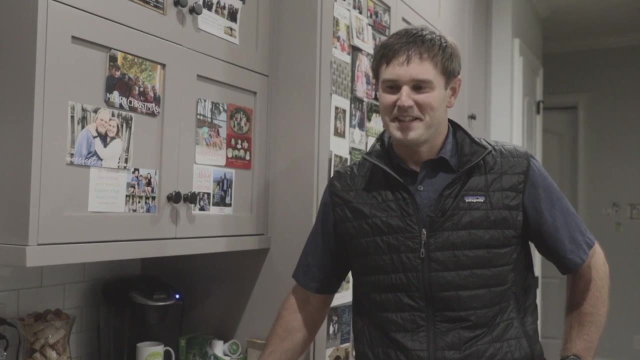 there's a lot of joy too. I don't, I don't mean to make it sound abysmal, It's fine. Well, I guess that kind of answers The next question. Why would someone not choose your specialty? Yeah, Yeah, So you know if, um, if you get frustrated with kids, if you can't hammer. 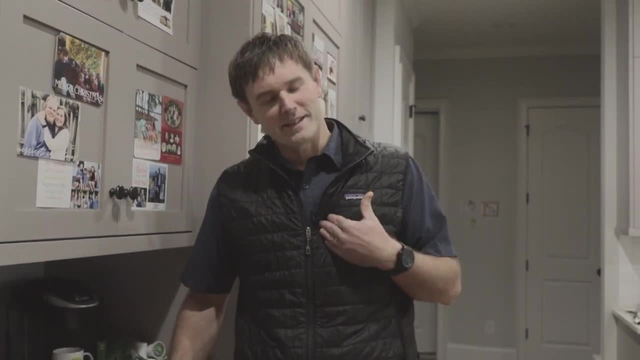 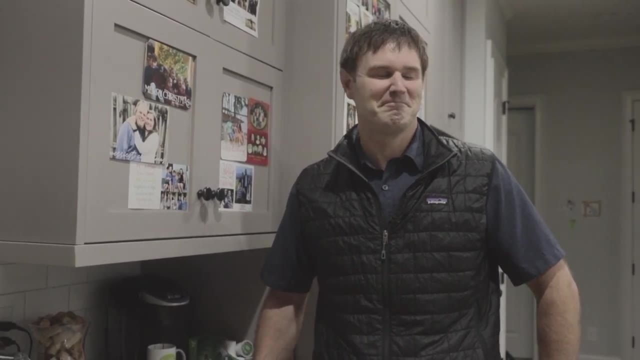 around with little little guys. um, if you have trouble getting you know back down to that level, um, you have trouble getting on your hands and knees and and, uh, picking up kids. um, you probably want to stay away. 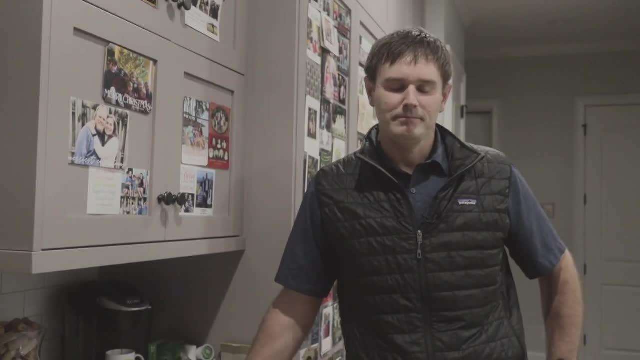 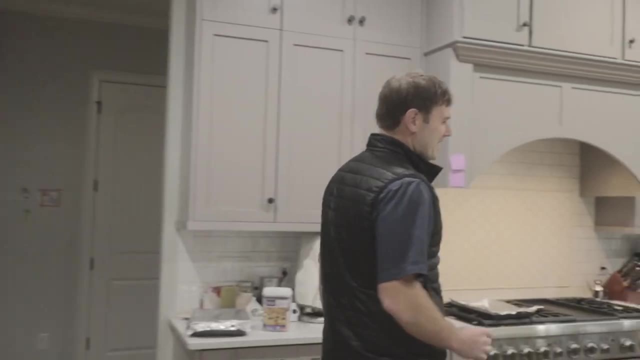 Well said, Are there any stereotypes of your specialty? Um, you know, I think probably one of the biggest stereotypes of our specialty is that just kind of softies, um, or maybe we're the nice guys. Um, I think that was the that. 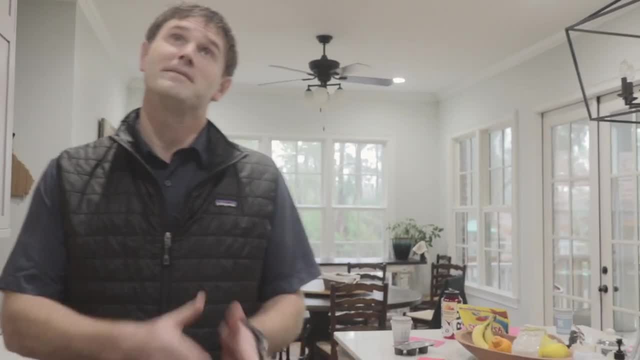 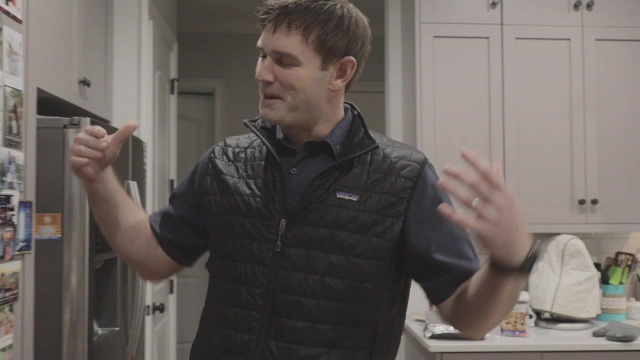 was certainly what we thought of the pediatrics residents, uh, residents and the attendings when we were rotating through pediatrics when I was in medical school. is that, you know they weren't the, they weren't the ones who were, you know, um, making you feel really. 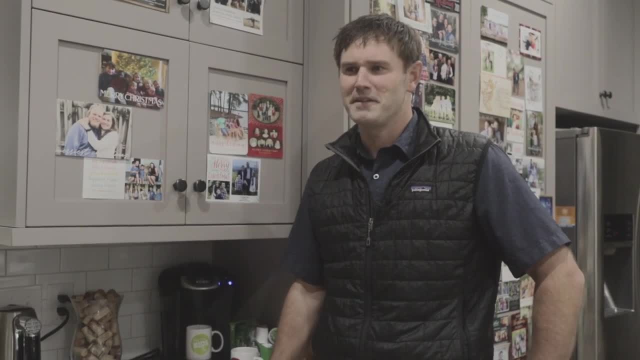 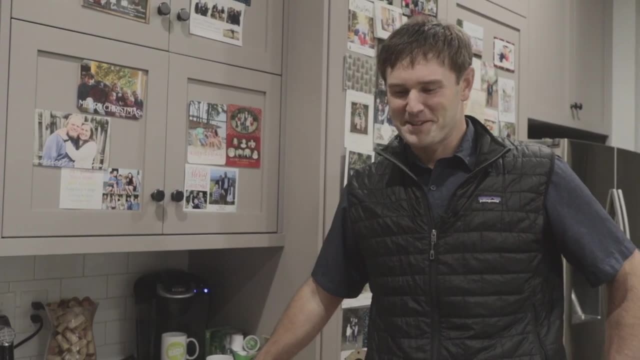 bad for not knowing something you know. when they ask you questions, you know it seemed like they wanted you to learn and not just this vindictive spirit. you know um like on a surgery rotation or something and um not to speak ill of surgeons, love the good. 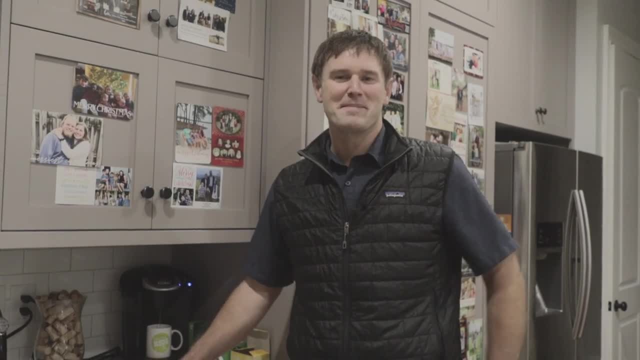 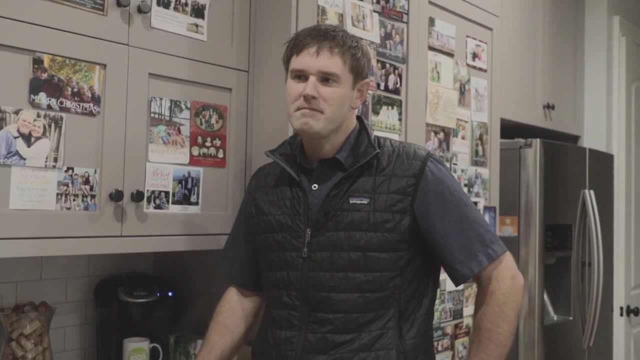 surgeons, you know, Um, but yeah, I think that's probably a stereotype. Yeah Well, would you say in particular, are the stereotypes true at all in your experience? Um, I mean, yeah, I think there's in general, I think probably the, the, the flavor of people. 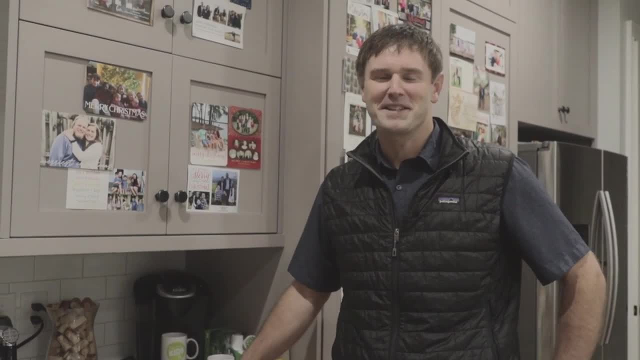 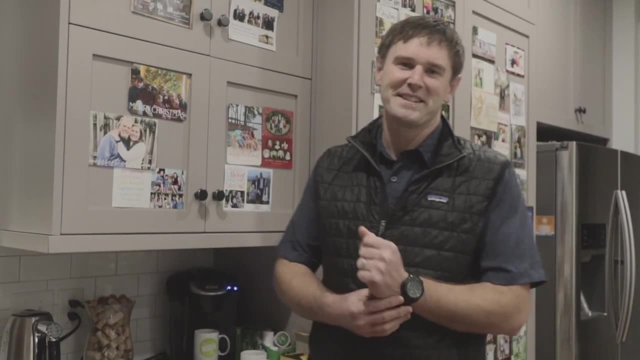 who go into pediatrics, um, are kind of natural softies, cause we love children and we want to. we're probably more gentle spirits and um, Um, you know, and that's not universal, but uh, you know sometimes, uh, you know you. 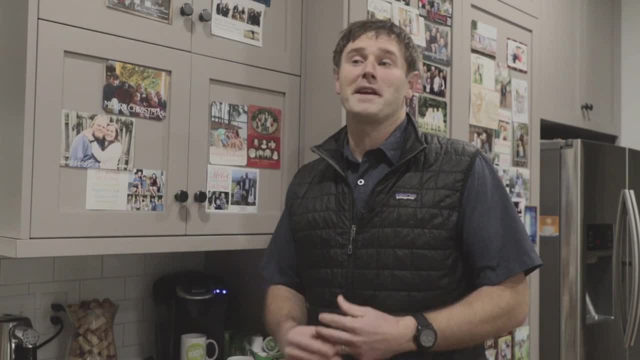 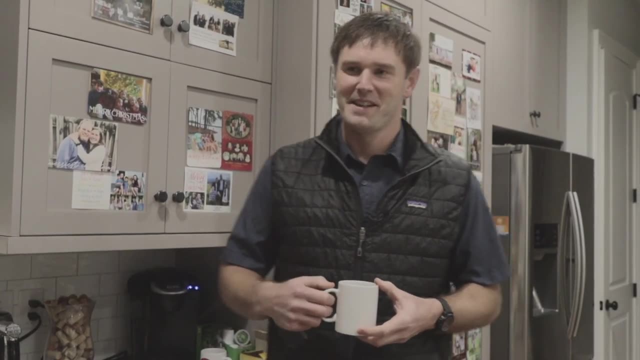 can you can be, uh, something. it's easy to provoke the anger of the, uh, the gentle spirits when you, when you, mistreat children- and you know we do get passionate about, um, you know, children, especially when they're at the victims of abuse and other things like. 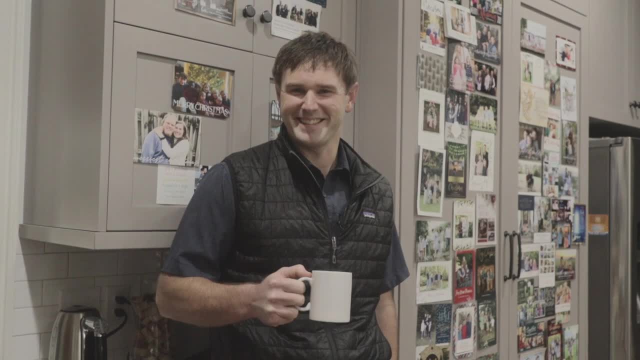 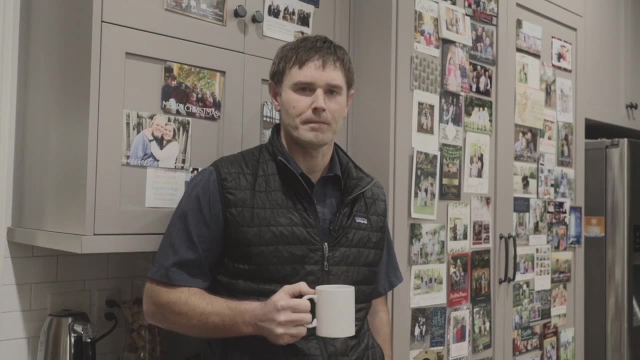 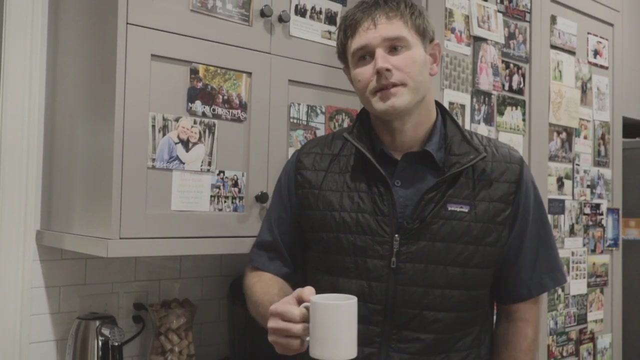 that, So we're not always sweet and kind. Well said Now, you touched on this earlier: even though you work in private practice, you are still able to interact with med students. What does that exactly look like? Um, so we actually interact with students on a lot of levels. Um, so, like we said before, 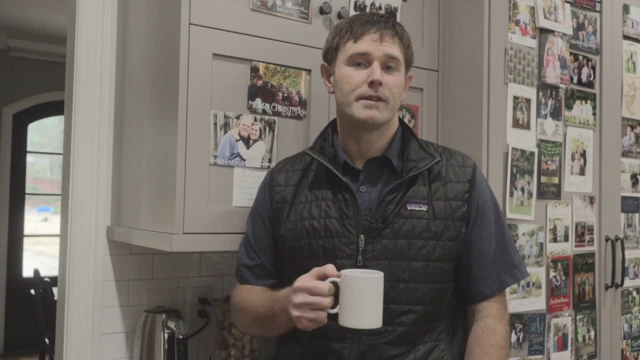 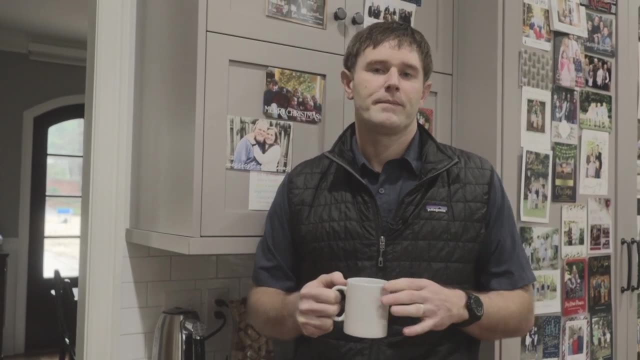 uh, you know, in the clinic um we take students um about every six weeks. we'll take students for a couple of week blocks and um they'll see patients with us and uh, we'll help in their training. 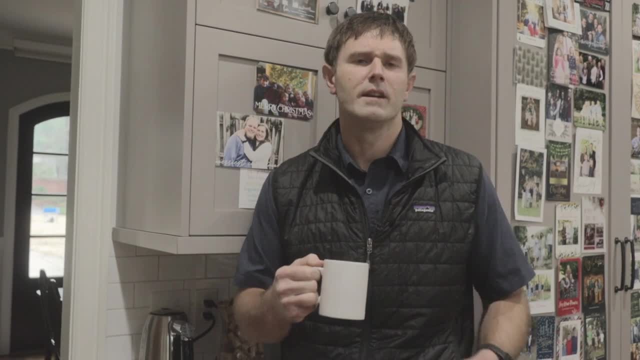 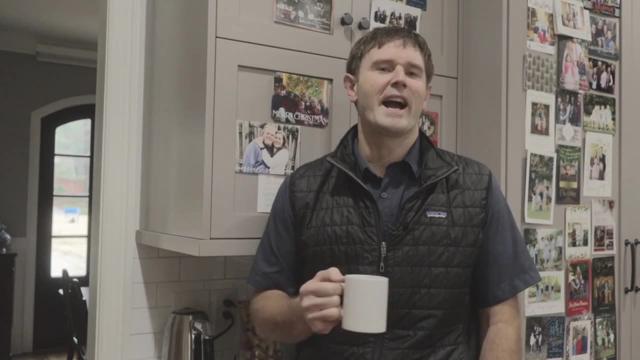 You know they'll. they'll make an assessment and we'll talk about plans, And so they're learning the ins and outs of pediatric medicine through the clinic, which is in private practice. it's a much faster pace than in the academic setting, Um, you know. so they get, they get. 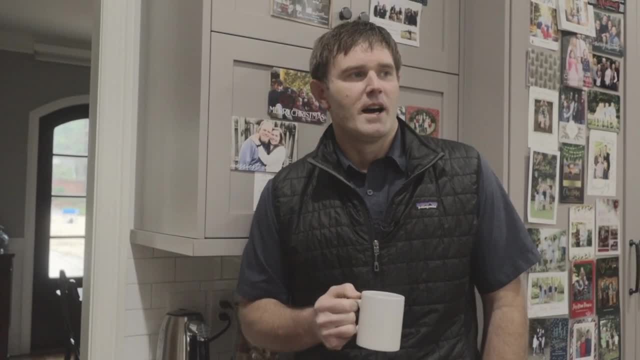 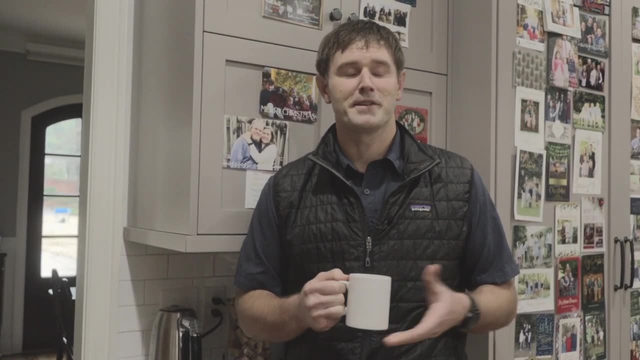 that flavor too, um at at our clinic. But uh, you know we we also do a lot of other stuff with students outside of um the clinic. Um, so we've been for years. we've been involved. 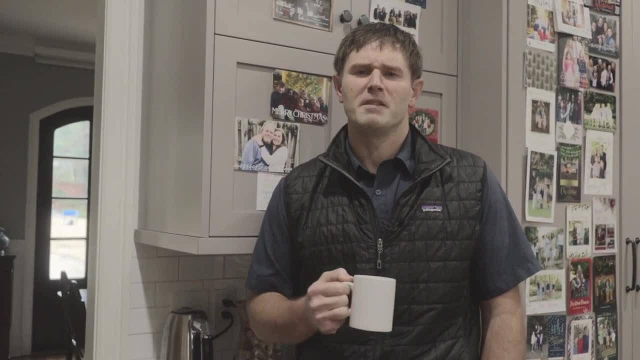 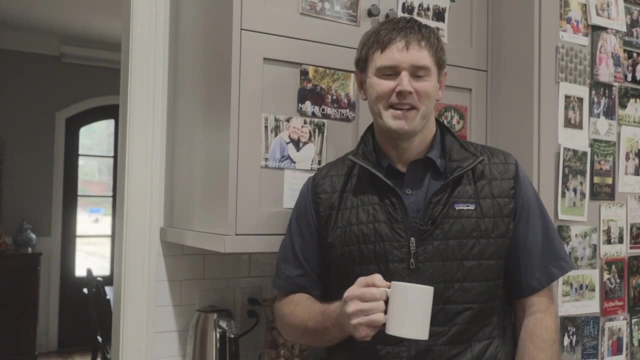 with the student, Bible studies and, um, you know, meeting with students. Um, so I've been involved with the students one-on-one a lot um, through various stages of their training. Um, you know, so I've I've really enjoyed having medical students. 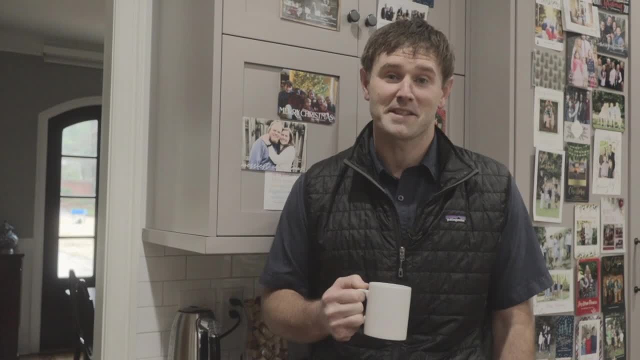 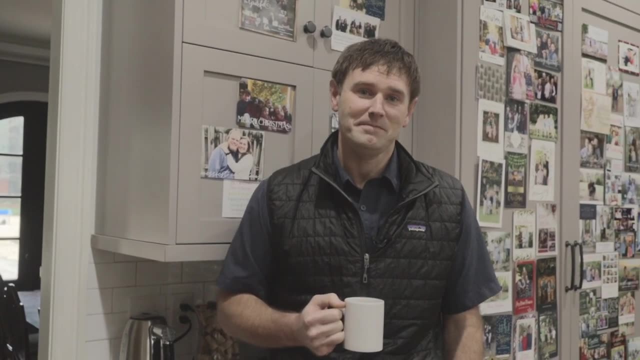 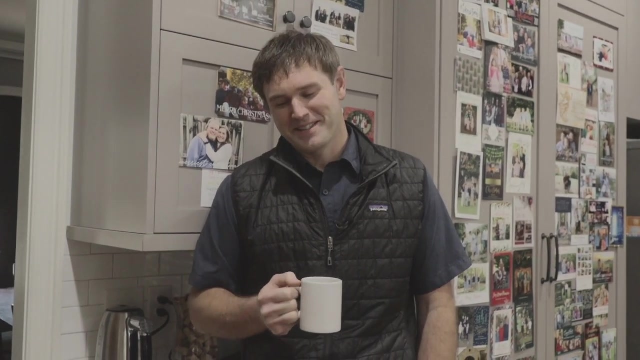 as a part of mine and my family's life um for the last really 15 years or so. That's awesome. Now some fun ones. What's the craziest question you've been pimped on? You know, I remember being on a uh trauma surgery rotation in third year medical school. 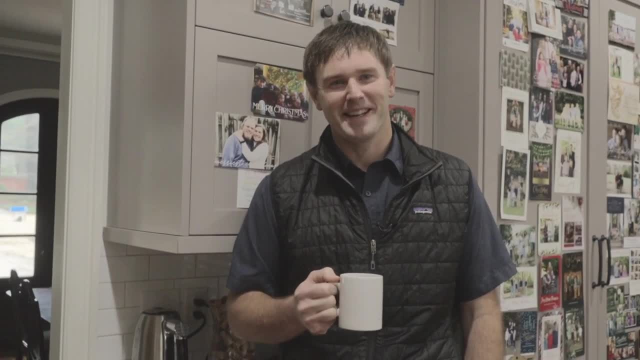 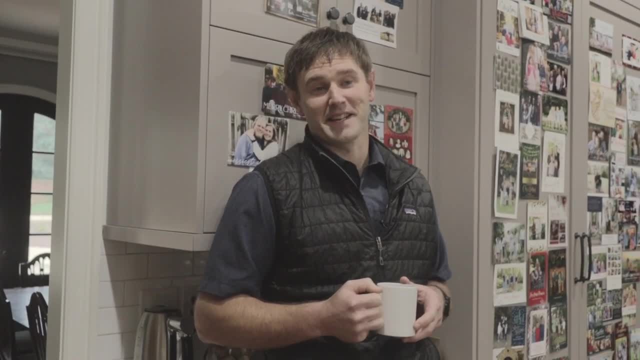 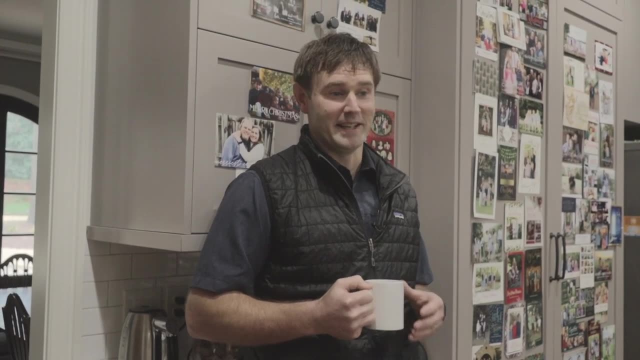 out of sleep for a um, a gunshot wound. Uh, this guy had several gunshots um, including one in the um inguinal area and uh which is kind of around the pelvis And uh the. 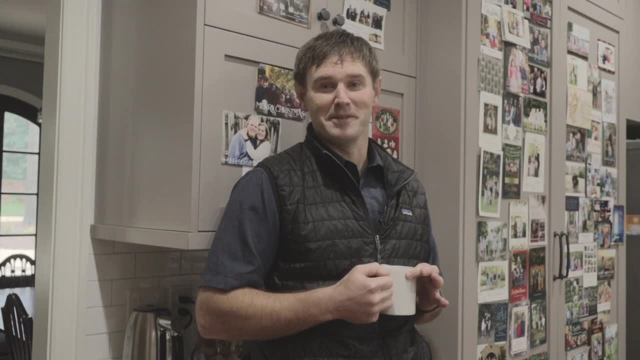 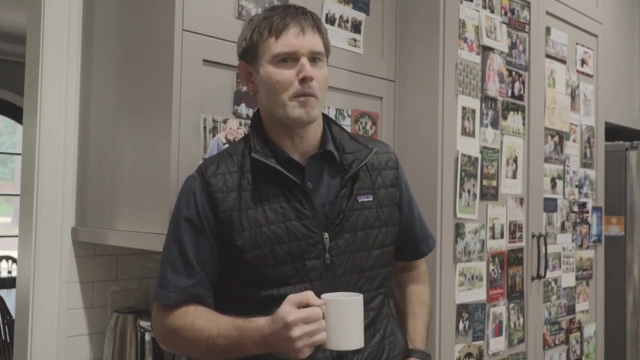 surgeon was dissecting and trying to find the bullet and he was screaming at me. you know what is the order of the. you know the vessels and the nerves and the uh uh around the femoral area And I'm stumbling through trying to remember the nerves and 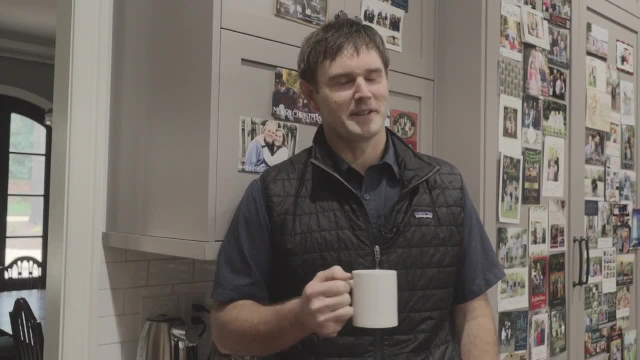 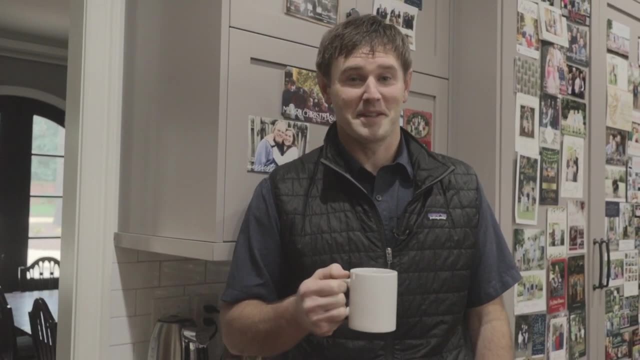 and and all the vasculature in that particular area and totally got it wrong. And it was partially because I probably should have studied a little more and, uh, partially because, man, he was hard. Um, but at 3 am that was a toughie. 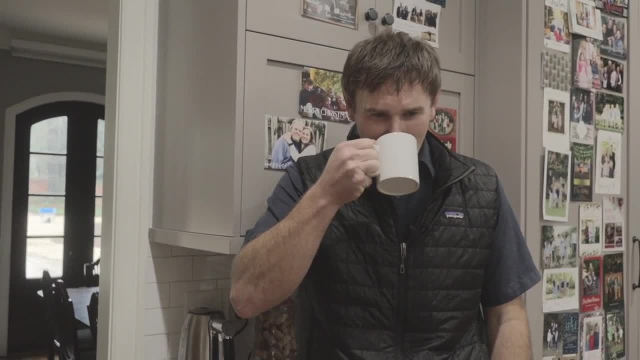 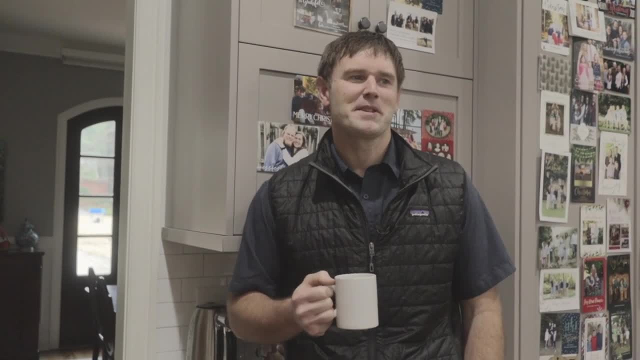 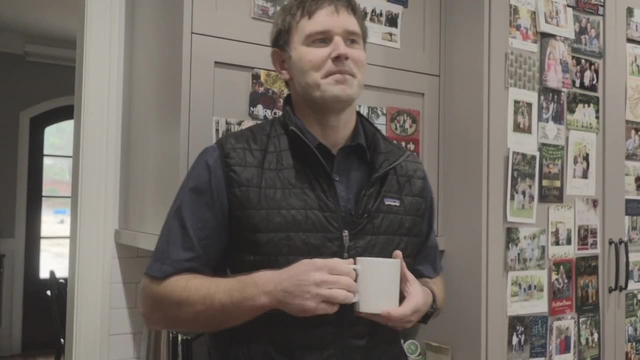 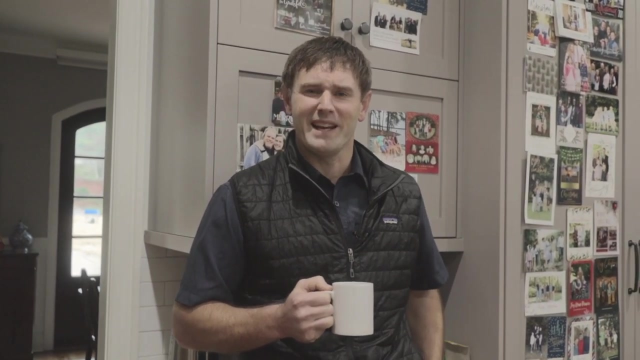 I think I'm. there's always a little bit of an anticipation. The starting clinic- um, usually our schedules are pretty busy and um, so you kind of see a kind of a mountain in front of you sometimes, um like ugh, how we're gonna get through, um, how we're gonna. 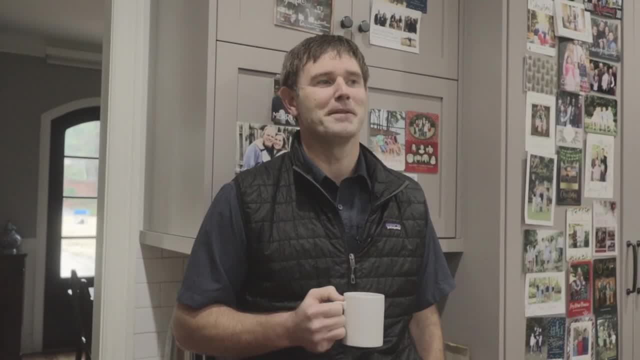 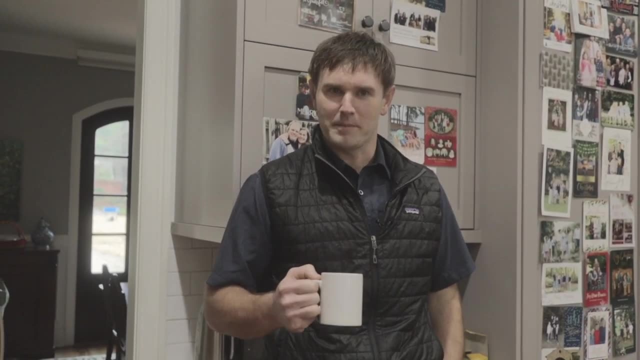 get through and take good care of these people that are coming through the clinic today And and you can always, you always look at our schedules and I try to make sure I um think about how I'm gonna time Dr. Yeah, on that side. 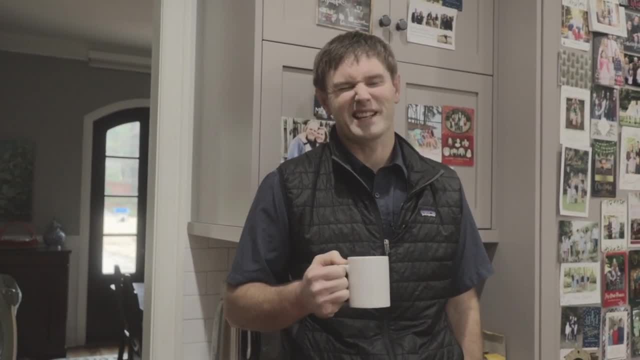 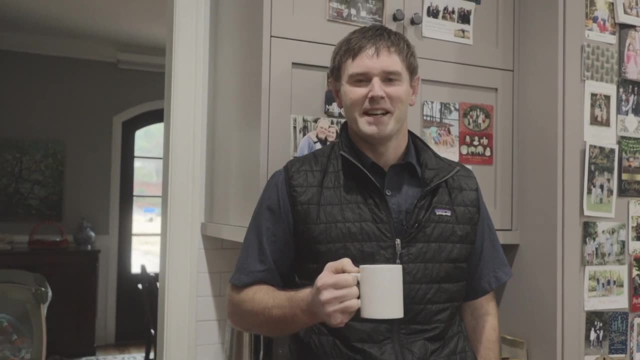 um visits, um, you know, because I just kind of anticipate some, some people needing a little more Um, and there's just always things that come up, Um and so, uh, it's just a little anticipation about how, how, how we're going to um make sure we're taking good care of everybody. 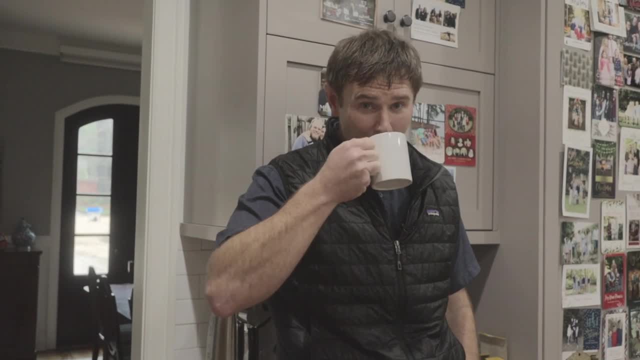 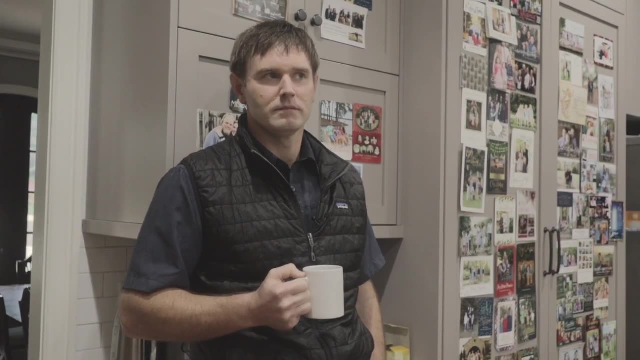 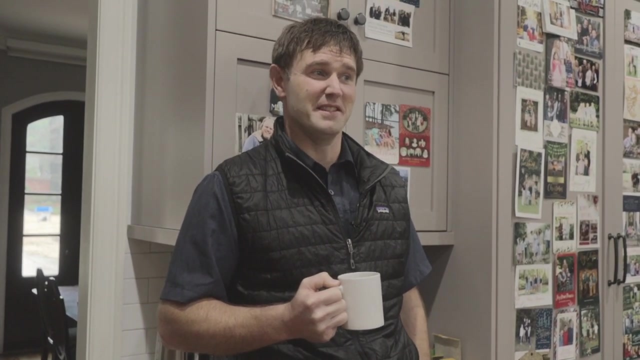 I understand. Well, all right, So here's some quick fire questions. How many patients do you see on an average day? Uh, 25 to 30.. What's the most amount of patients you've seen in a day? Ooh, about 40,, but that was. that was not good, I would say. seeing that many patients in one day is. 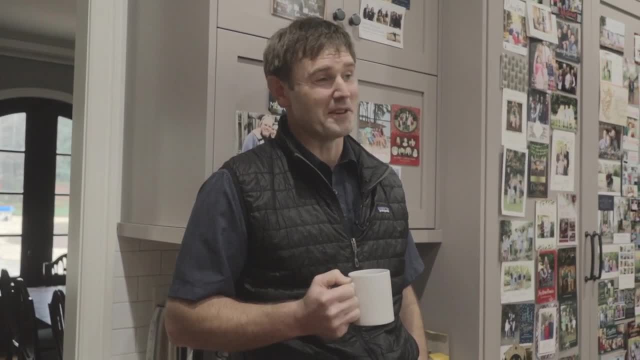 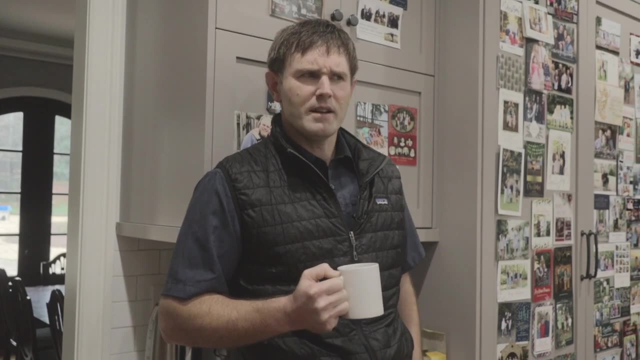 borderline dangerous, Um, and I don't know that you're ever really taking good care of people when you're seeing patients that fast. Do you ever have to do any procedures? Uh, simple procedures, Yeah, I mean, we, we do incision and drainage of abscesses. We'll 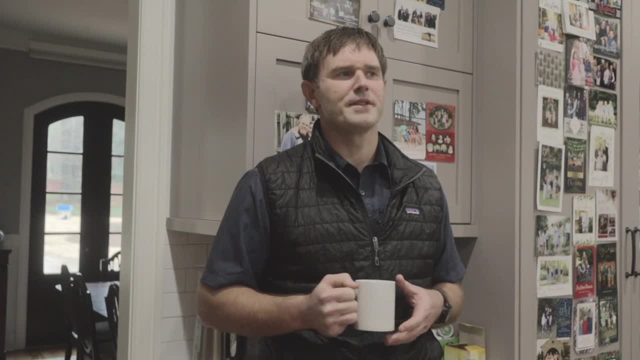 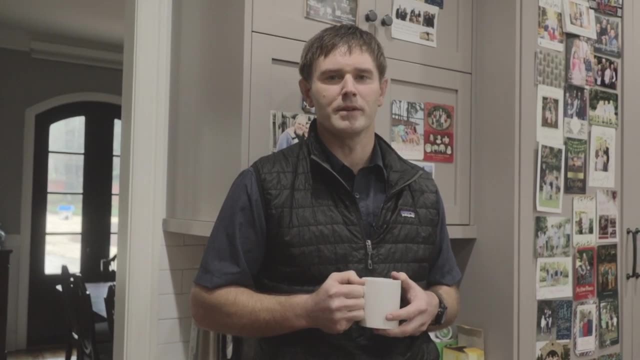 we'll do suturing um, mostly Simple sutures Um. so you know, anything that's uh severe um are going to be very cosmetically significant And we'll usually turf to uh the surgeons, the pediatric ER Um. 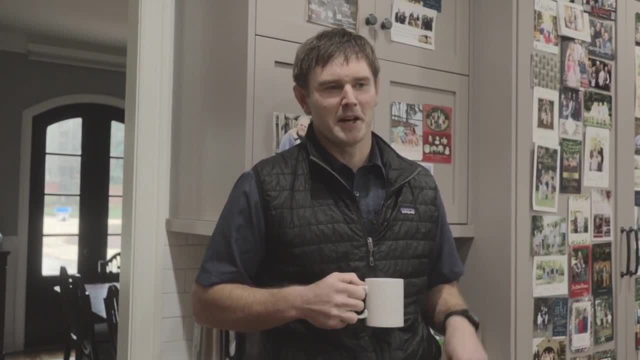 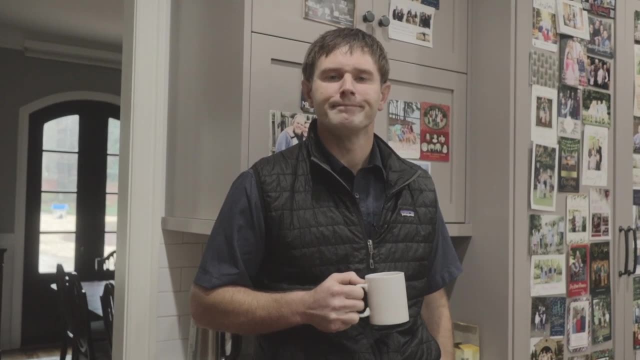 um, you know we'll, we'll clip, clip tongues um for, uh, babies who are tongue tied and need some help nursing. you know just simple procedures like that. Okay, How many hours do you work in an average week? Um so, actually I I work. I work four hours a day. Um so I work, I work four hours a day. Um so I work. I work four days a week, um plus the call we take. Um so, but those days are usually long days, They're. usually 10 to 12 hour days. Um, so usually between 40 and 50 hours a week. What time do you normally wake up? Um 530 to six. What time do you normally leave the clinic? Um, on a good day I'm leaving around six. Um, on a real busy day, it's closer to 630 or seven. 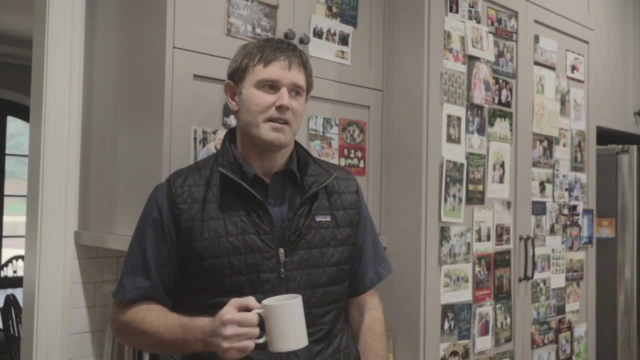 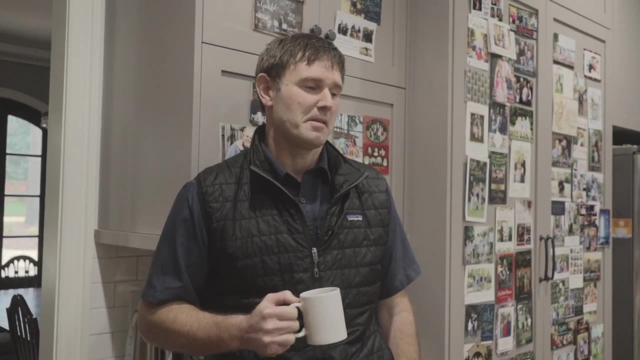 Okay, How many hours of sleep are you typically working on? Um six to seven, Okay. How many hours of sleep are you working on right now? Yeah, probably seven. Okay, My wife went to breakfast early with a friend, and so daddy was alone with the kids this morning. 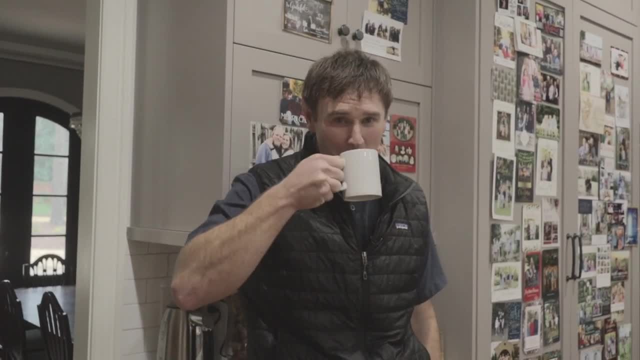 That's a good day then. How long did it take you to finish your patient notes at the end of the day? I do my notes as I go along. Um, so I don't. I don't try to tie things up at the end of the day. 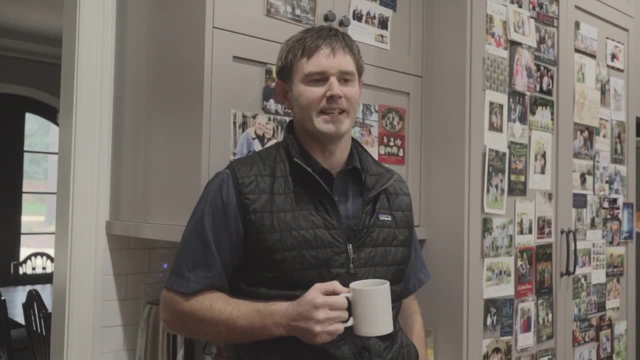 Um, it takes a little bit longer in the room, but, um, I feel like I'm fresher and I'm going to write a better note If I'm doing it with each patient. So who are you most thankful for in your care team? 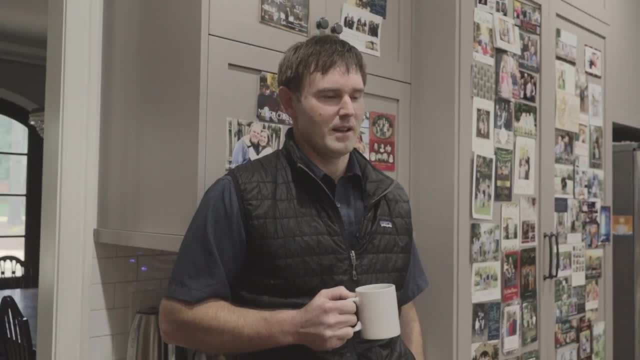 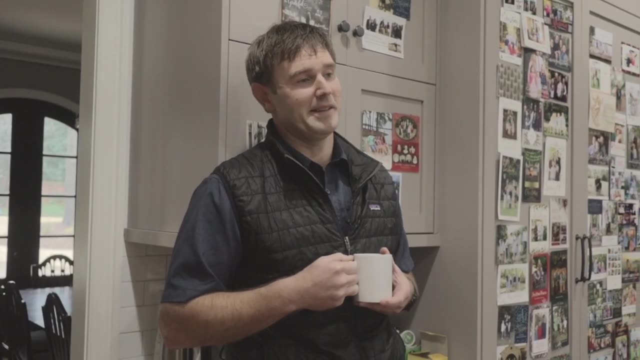 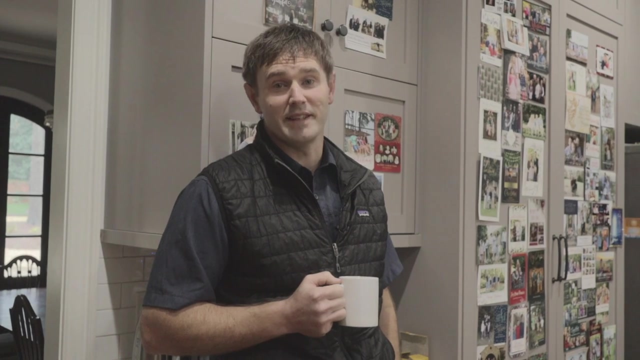 Whew, man, Um, that's a toughie, but uh, you know, I would say, uh, my nurses, um, you know the nurses. having a good nurse, um, is one of the most valuable assets that anyone can have. 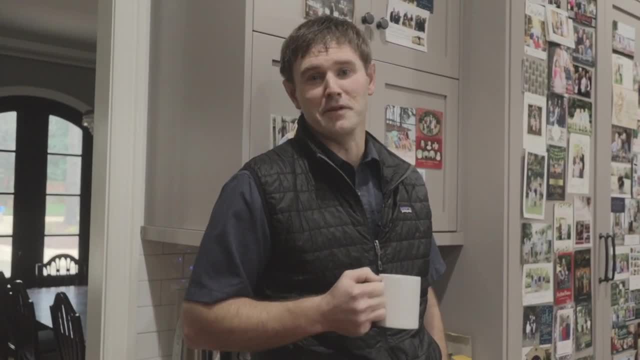 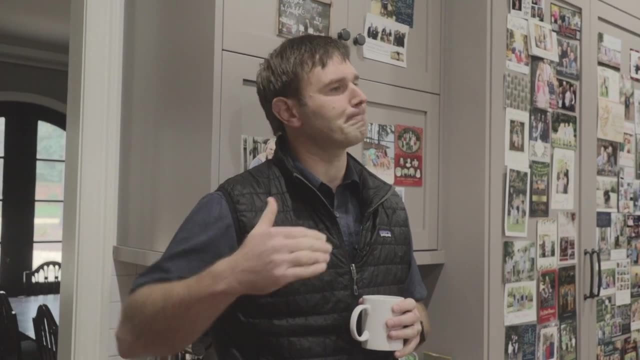 Um, as a physician, um, a nurse that can anticipate your every move, um is is really Just, um, you know, kind of helping you, uh, to manage your schedule. Um, so I have several great nurses and um, so I'm really thankful for them. 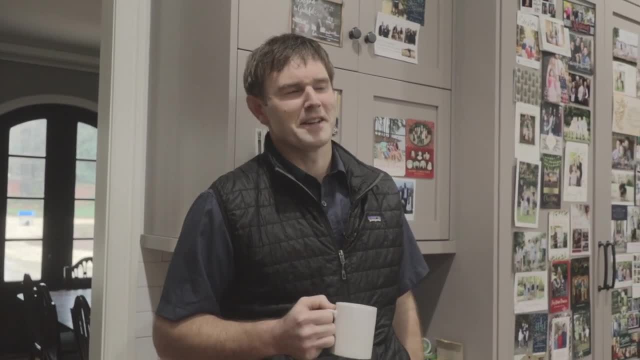 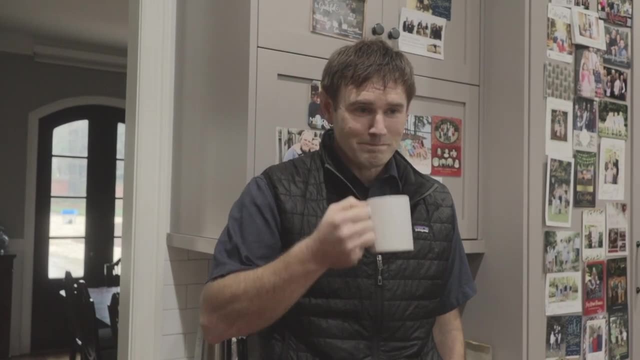 I have really good partners too, so I don't want to say, uh, not say too much about them. All right, Too little. So what's the funniest thing you've seen in a patient chart without you know, violating HIPAA, of course. 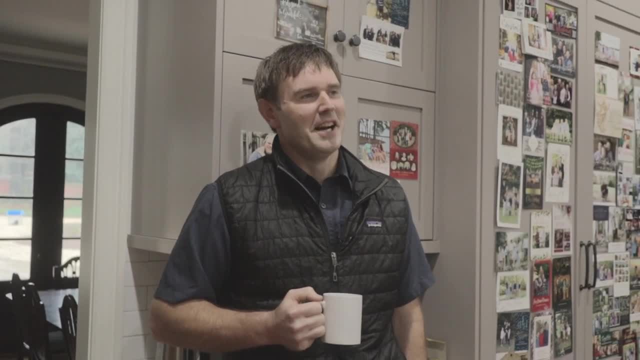 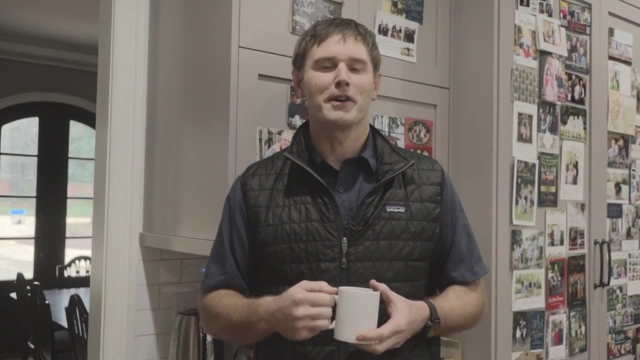 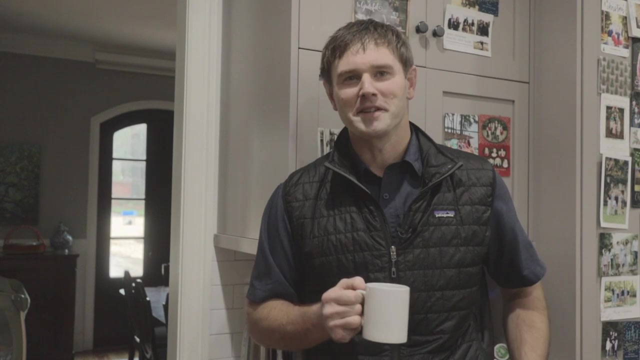 Whew, Um, you know, sometimes we, um, you know, we get records from other physicians when patients, you know, transfer, you know, or when they move and come to find a new physician. so you know, sometimes with these EMRs it's really easy to click, you know, yes or normal on the exam, and so 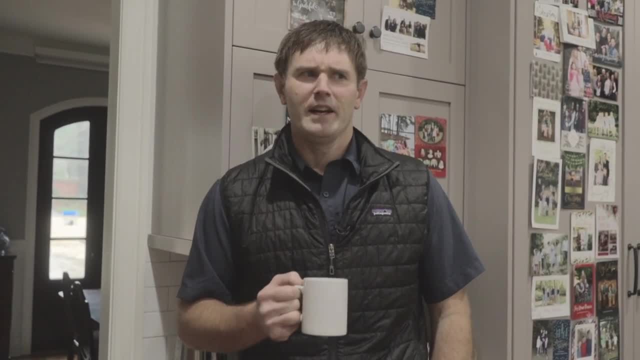 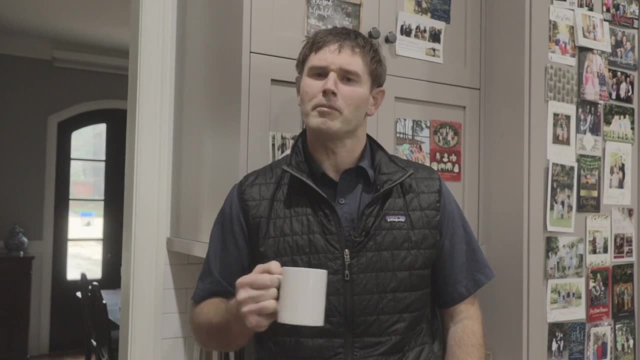 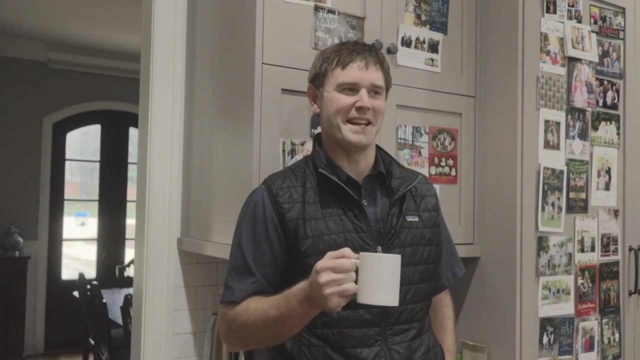 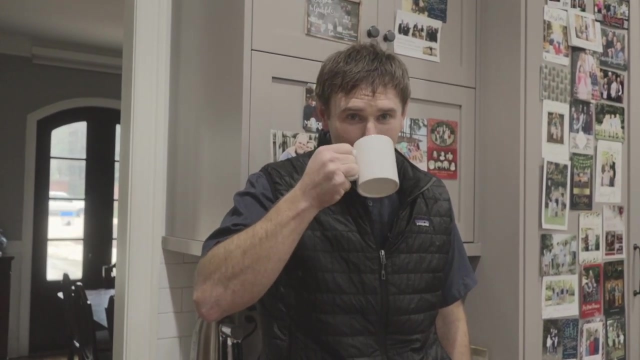 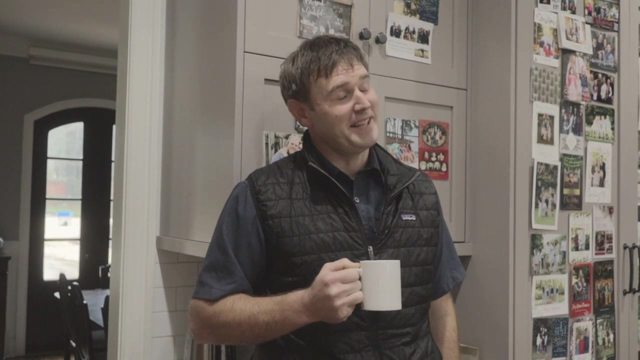 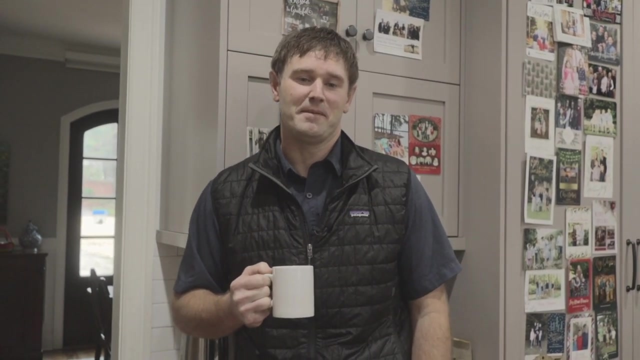 there was one position in particular that I've noticed that every time I saw a chart that came from that office, even the two-month-old males seem to have normal prostate exams and I thought to myself: probably, probably a very small chance that she did a prostate exam on the two-month-old, but that was pretty funny, all right. so what's the most common medical advice you give to your patients? you know that that's a hard question because I give a lot of advice on a lot of different stages. you know, I think probably one of the most 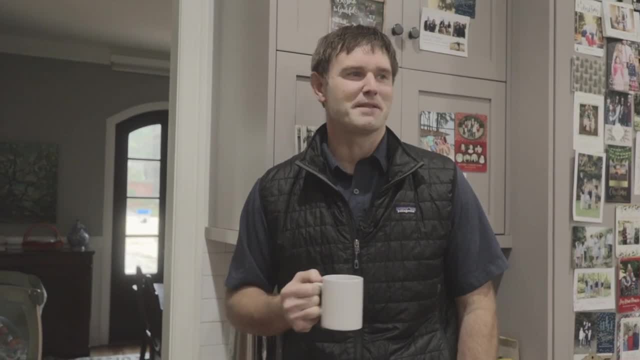 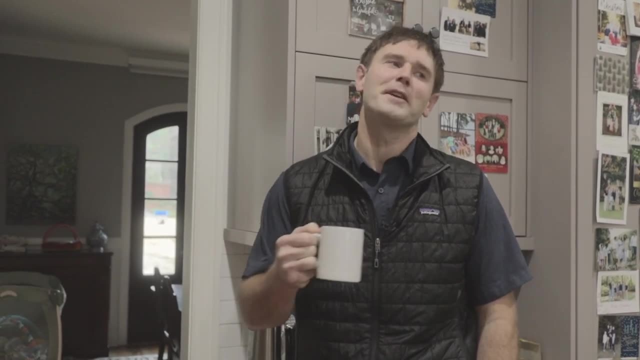 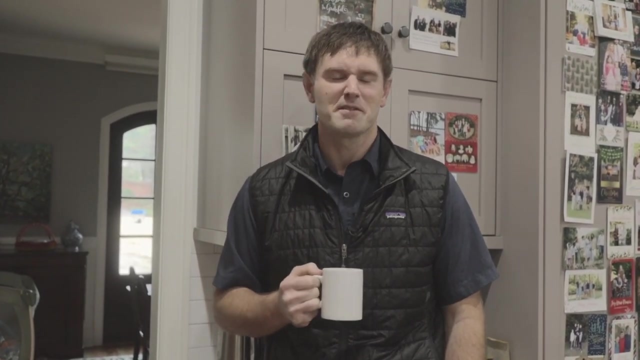 frequent advice I give to parents is especially parents of toddlers- is just, you know, try to be consistent with your children and be as good at encouraging them and affirming them as you are at correcting them, because children really need both. they need consistency with affirmation and also correction, which 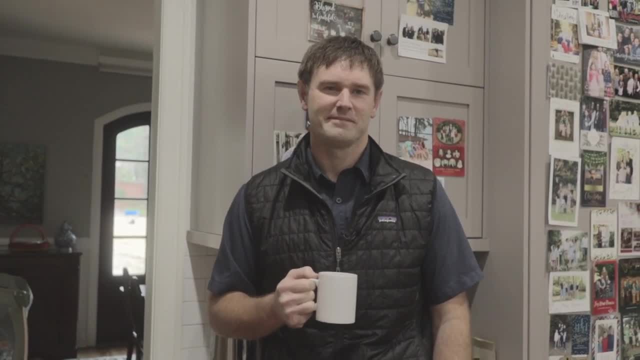 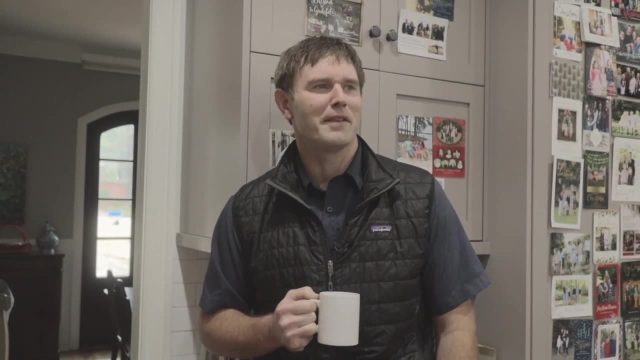 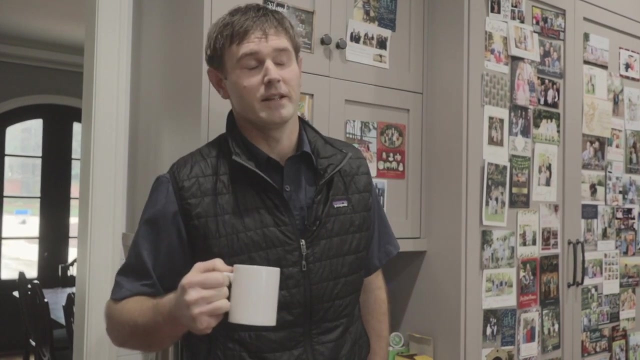 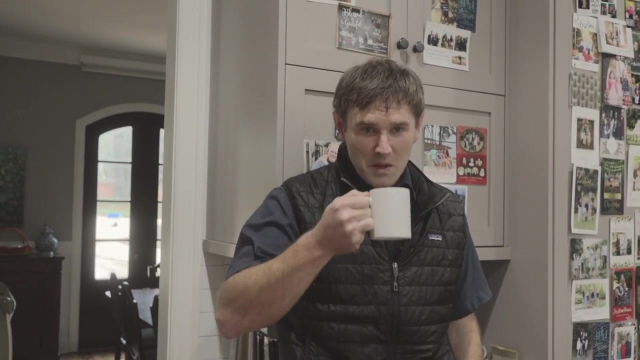 isn't quite as fun. well said, what's your favorite nerdy random medical fact? if you have one nerdy random medical fact- I don't know, I'm sure that I'm a nerdy random medical doctor, but we can come back- so and then, yes, you know, we typically can't avoid talking about it. 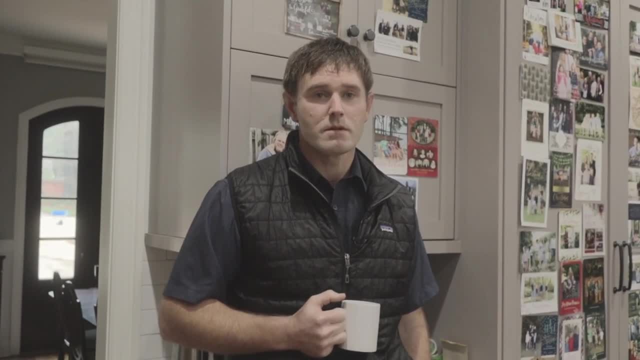 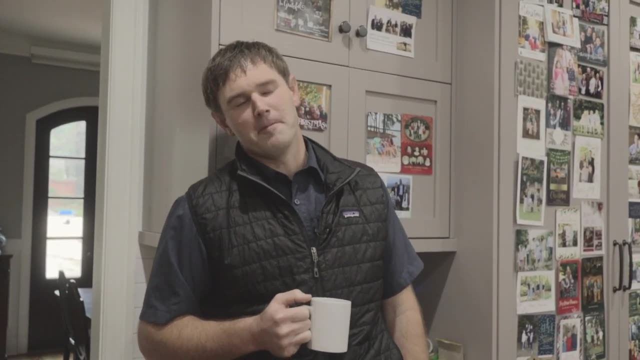 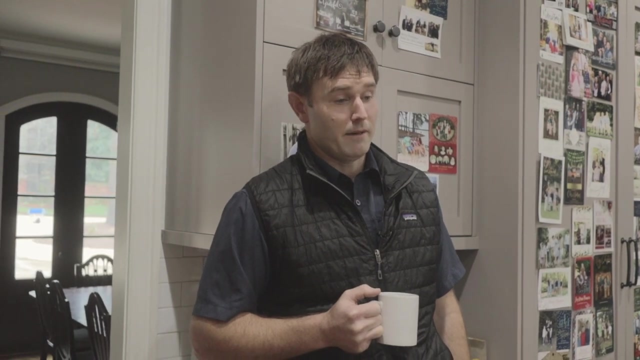 right now. but how has your clinic, and your specialty in particular, been impacted by COVID? yeah, so COVID brought a whole lot of unique challenges, that's for sure. you know. initially, when COVID hit back in March of last year, our volume, our patient volume, went way down. you know a lot of it was just 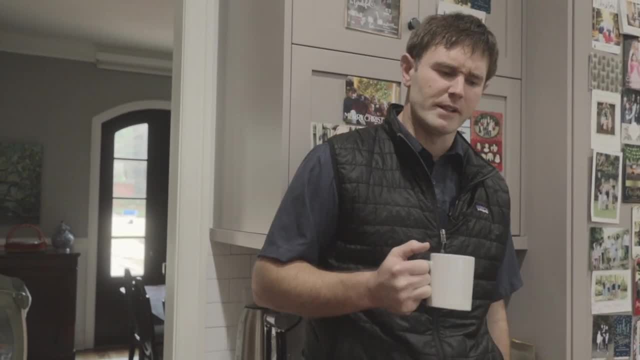 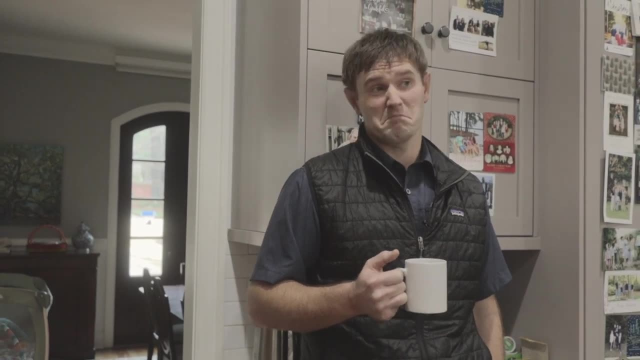 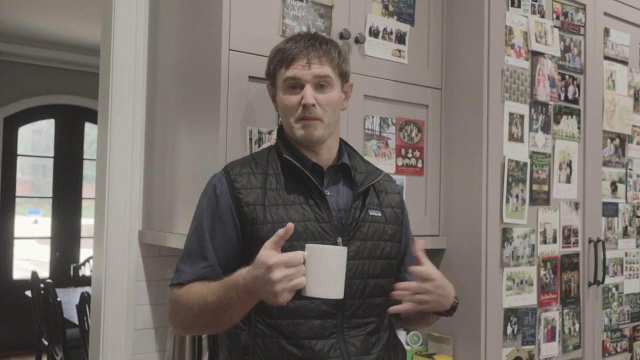 people, you know, sheltering in place at the time. a part of it was that they're just. as the months rolled on, we just didn't have any sick patients, which was, you know, that's a really good thing. actually, people were, I think, either staying, you know, being careful about washing hands, and you know they just weren't getting sick because they weren't around each other. so patients weren't getting sick and they weren't feeling well. and also, I think a lot of people started weighing a little more, like what's worth going to the doctor for? do I, do I need to go to the doctor for this or so? there was a lot, you know. 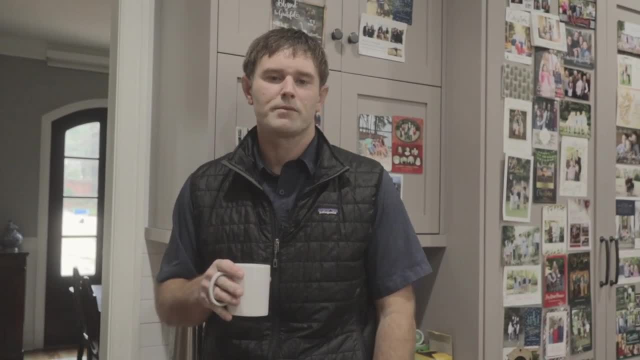 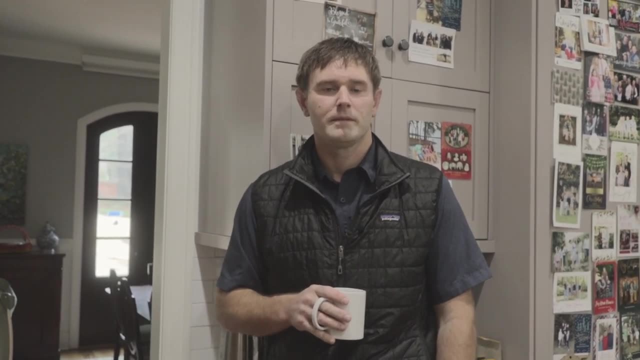 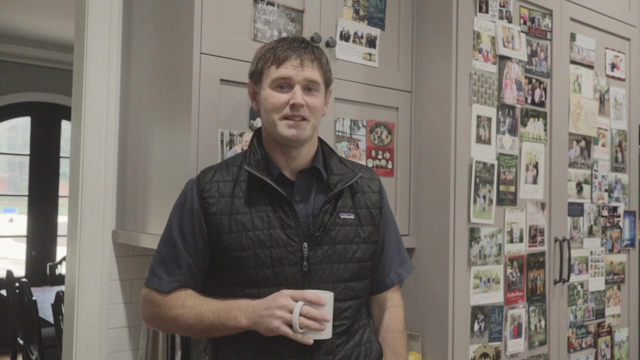 less of just the simpler stuff, which we're always glad to see, but it's really cool when parents are feeling comfortable to take care of themselves too. so we've talked a lot about your life inside the clinic and in a clinical setting. how about your life when you clock out? so what is your favorite thing? 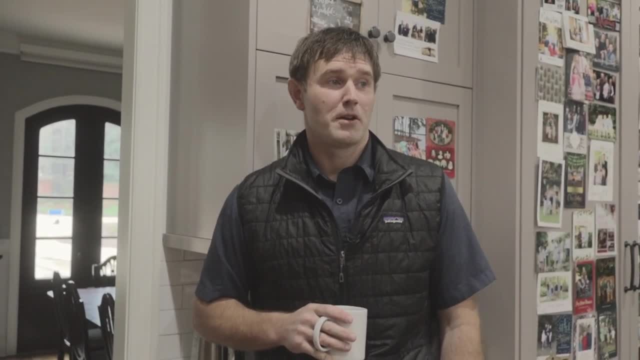 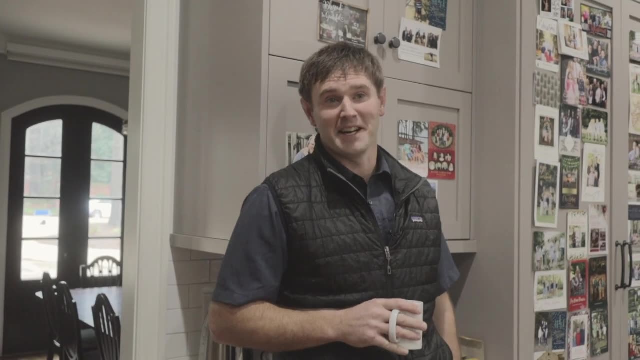 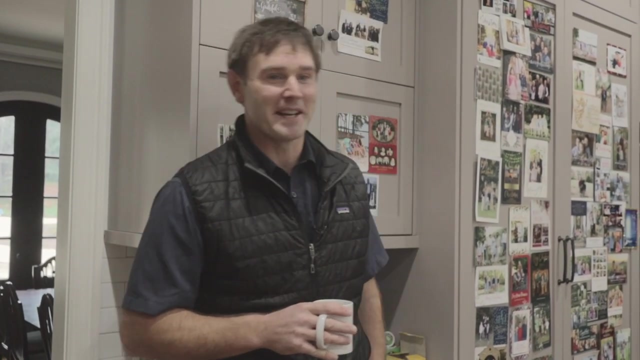 about working. wow, so if I'm not working I love to be outside. I mean, that's kind of my anything outside. right now there's a whole pile of wood in the back to use a chainsaw and chop up and split with an axe. so we like doing that, my, some of my. 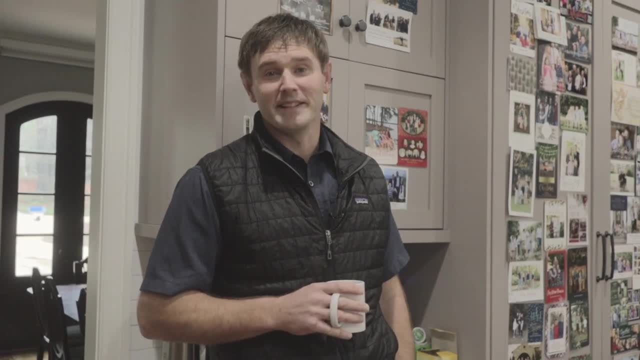 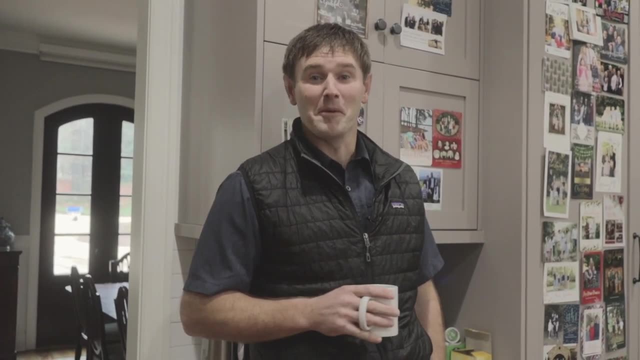 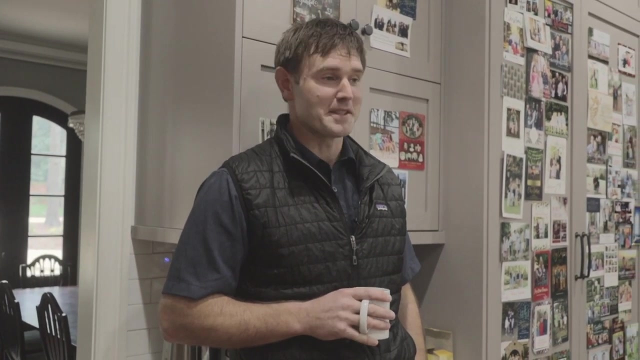 boys like to do that with me. I love to go hiking and, you know, be in the mountains, so that's kind of if I, if I had infinite time, I would probably do a lot more of that. so you have any kids I do. I have eight children actually, which I guess is. 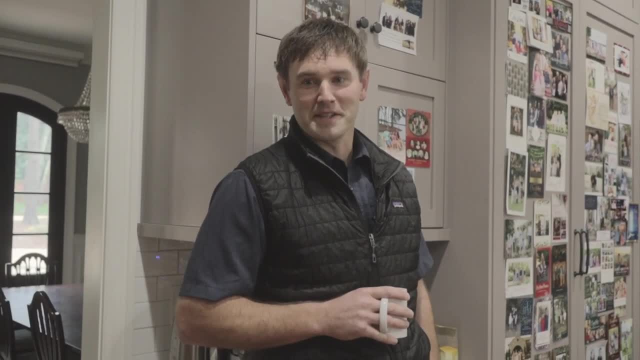 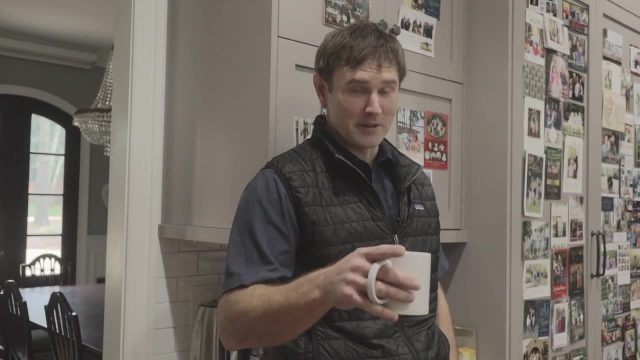 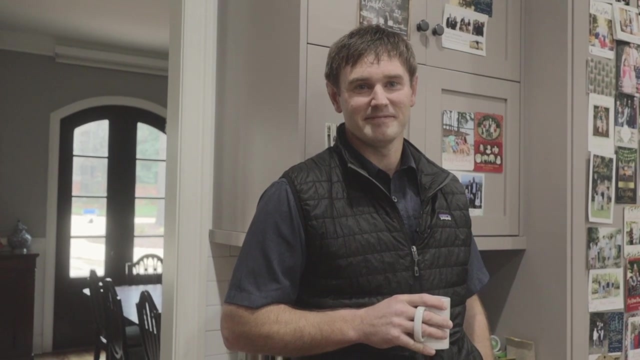 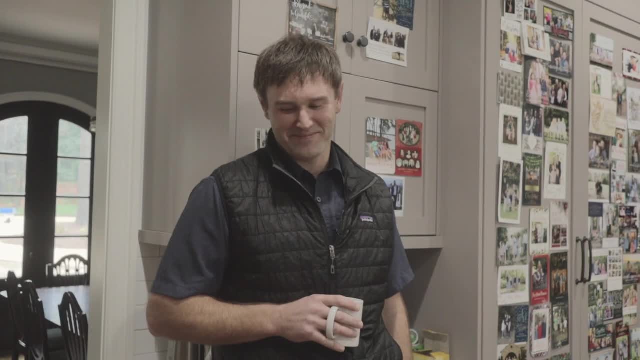 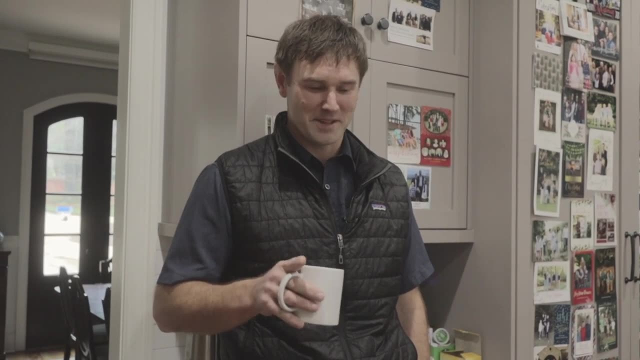 doctor and I became a doctor in my family's eyes and even even now I'm getting almost daily texts about my dad who's in the hospital right now for a non-covd- thank the Lord- a non-covd related issue, but I'm getting having to. 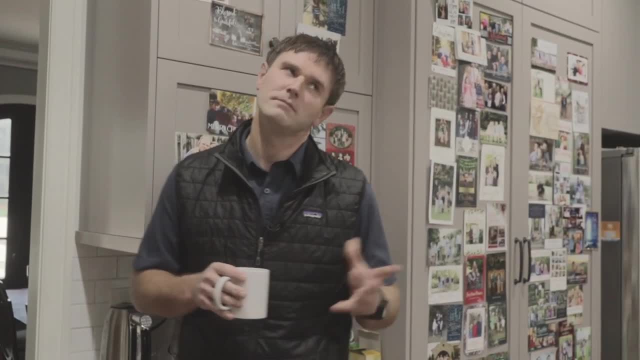 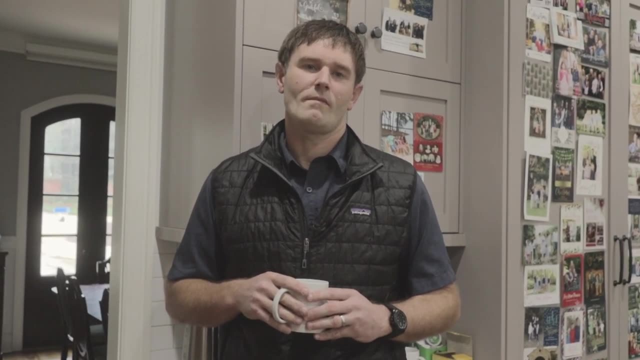 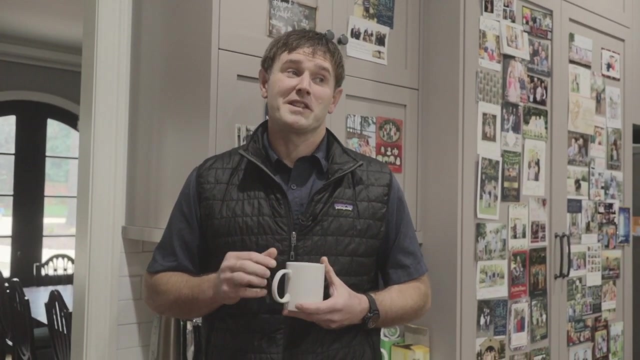 interpret some, some of his lab work and whatnot, which I'm mostly qualified to do, I guess yeah. so with that, what's the weirdest question a family or friend has asked you? you know I don't know about the weirdest questions, but I do get some really weird. 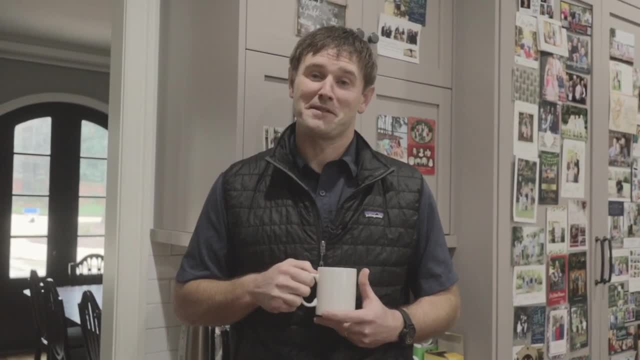 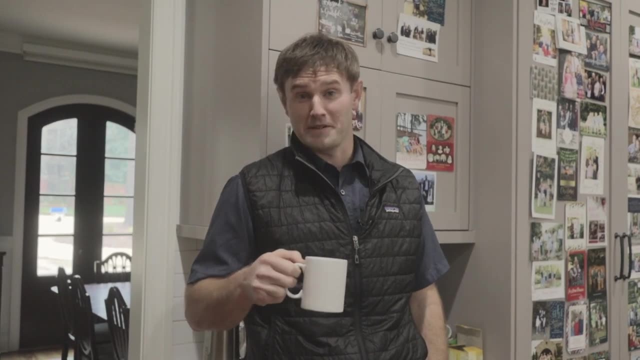 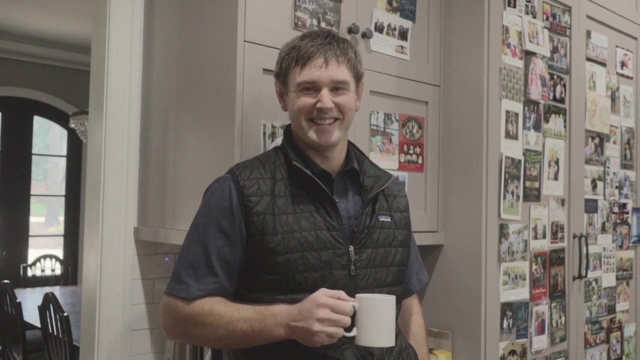 pictures. you know, like I'd have to, that I pretty much have to immediately delete once I look at them- from families and friends who have concerns particularly about. you know various types of diaper rashes, so you can imagine it's. it can be a little little wacko. my phone, yeah, pretty. yeah, you have any pets not? 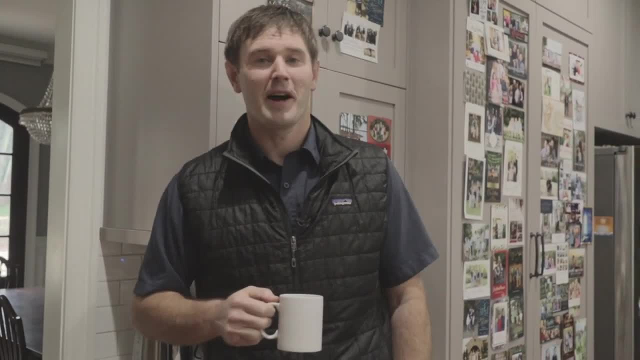 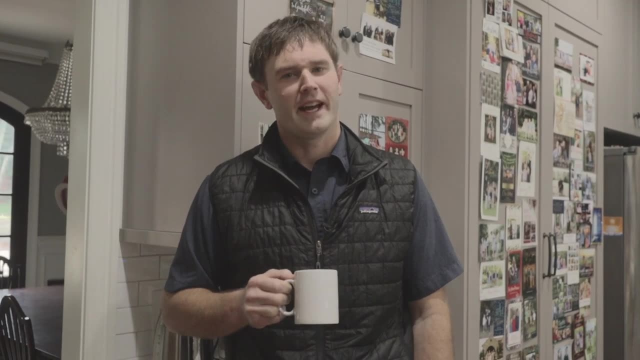 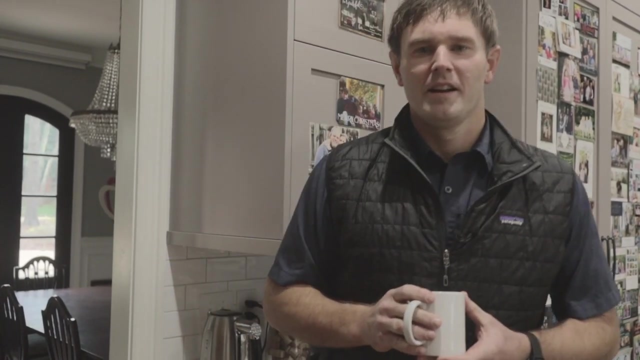 anymore. we, we had a dog for a while that he went to live at the grandparents house, but we won't. we want another dog and our cat, I think, got assaulted by a fox. well, let's say, are you a dog or a cat person? that I'm a dog person. yeah, the cat, you know. 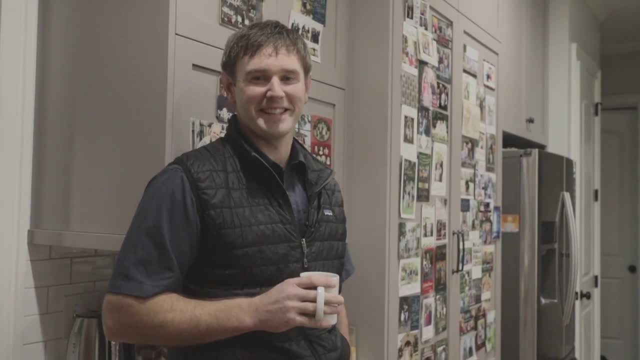 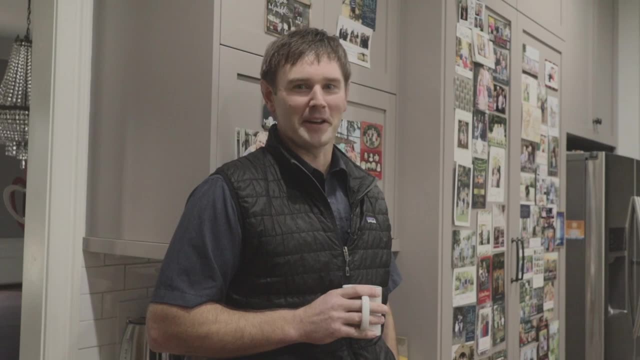 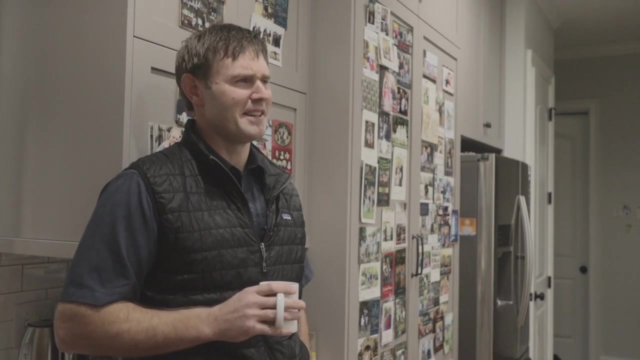 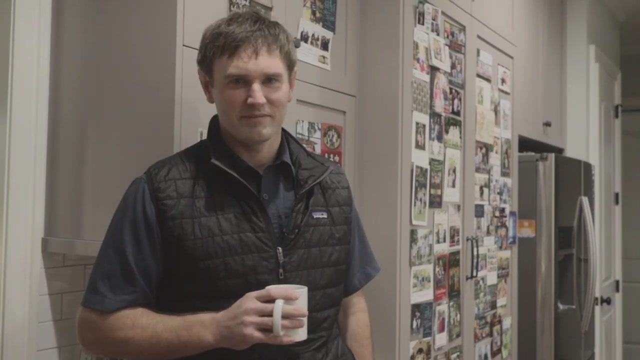 he can rest in peace. favor, animal, not a cat or dog. oh, hands down, it's birds of prey. They're- probably they have to be- the most amazing of God's creatures. I mean to watch something that big take flight is unbelievable. If you could have dinner with anyone in history, who would it be? 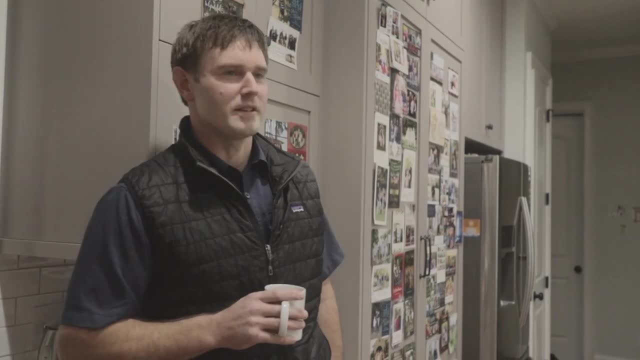 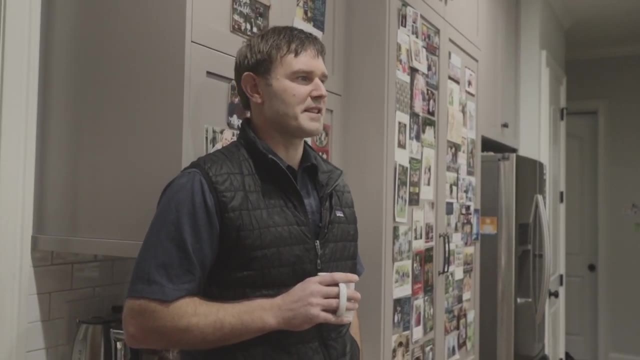 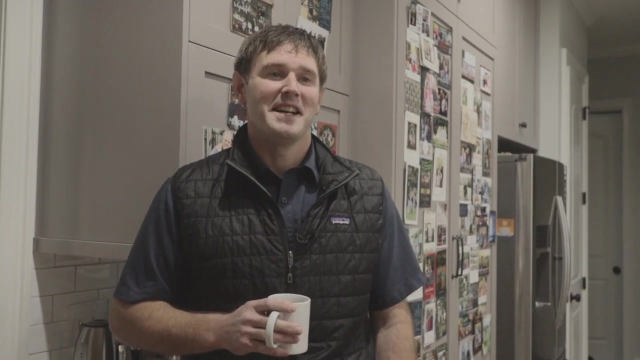 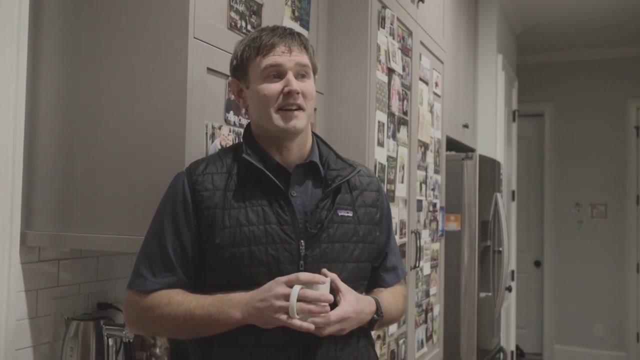 That is a hard question. Anyone in history. You know I mean that's a toughie. You know I mean certainly Jesus would be probably the best guy Since he wrote history in general. But I think if you're talking about just a man, somebody I really respect is a guy named Dick Winters. 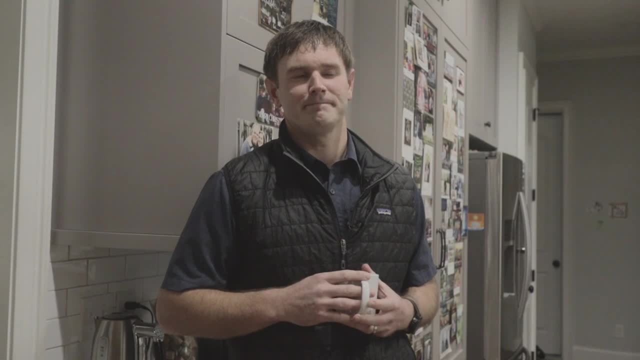 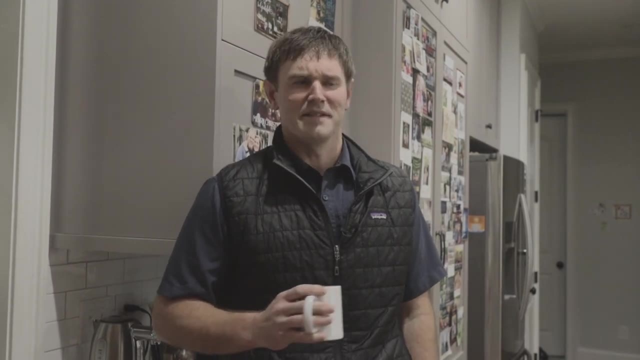 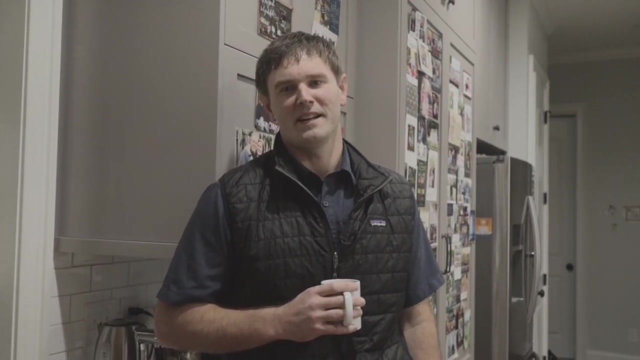 He was the captain of the Band of Brothers from that series. If you've ever read the Stephen Ambrose book, he just lived this incredible life And was a man who knew how to lead men, who knew how to sacrifice for others, And he just passed away a few years ago. 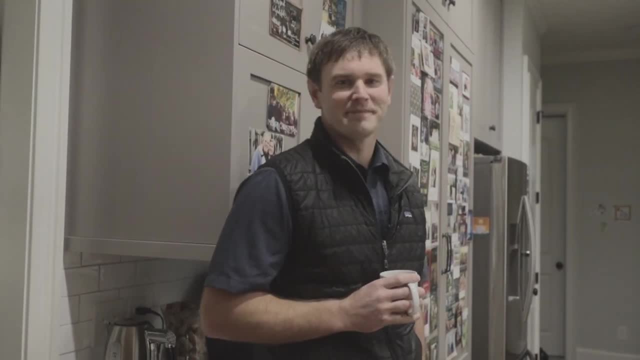 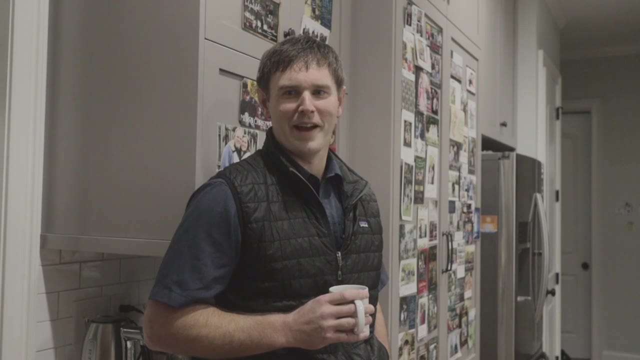 But I always thought he would have been a great guy to sit down with and talk to. Well, at that dinner, what do you think you guys would be eating? Definitely steak, A nice fat ribeye steak. What's your favorite dish to eat? 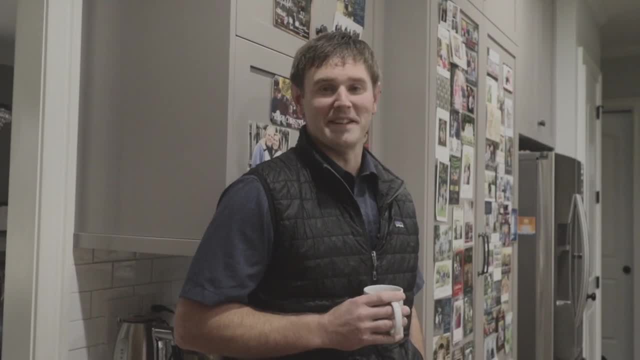 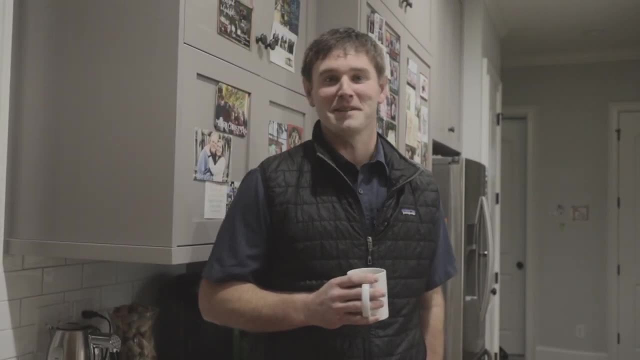 That might have answered that question. Yeah, it'd be hard to beat, that that's for sure. Any favorite restaurants around here- Well, I mean for my money, Frog Hollow Tavern- There's probably not a lot of places. There's probably not a lot of places that can get better than that. 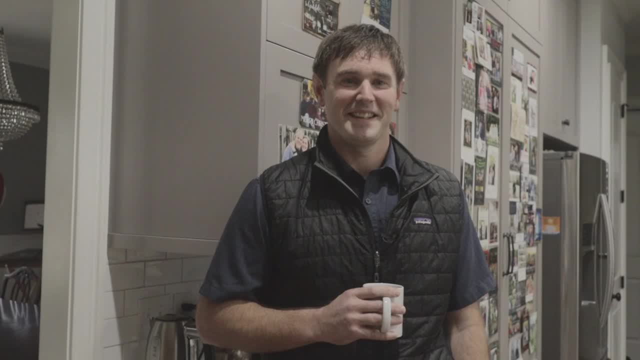 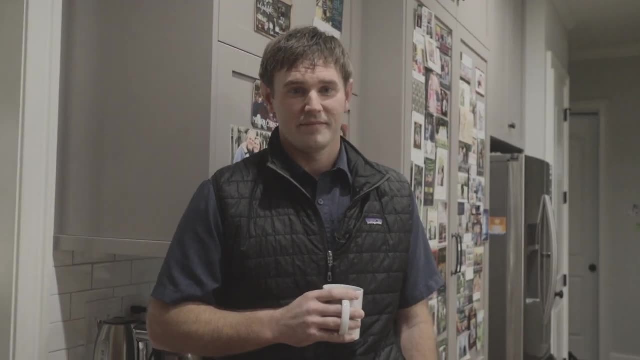 That's free advertising. I'll have my people reach out to their people. So, coffee, tea or soda Coffee, How much water should you be drinking every day? Eight cups. I don't usually get there, but I should. 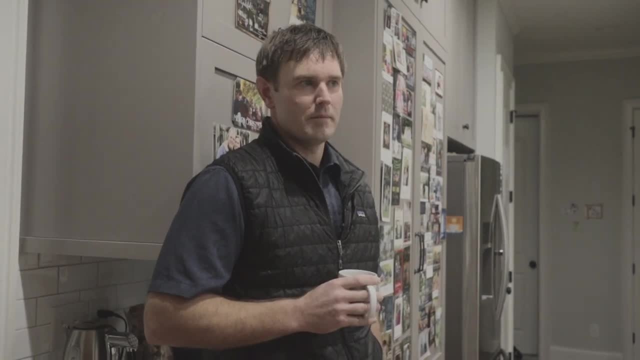 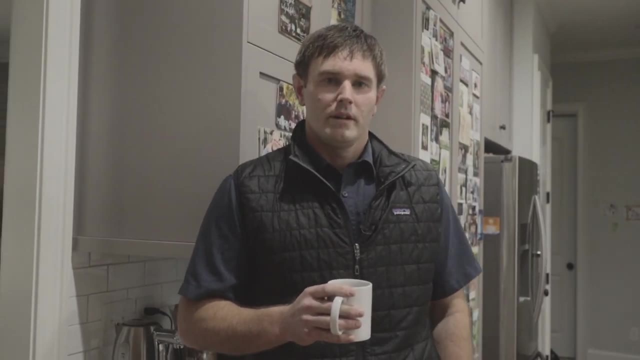 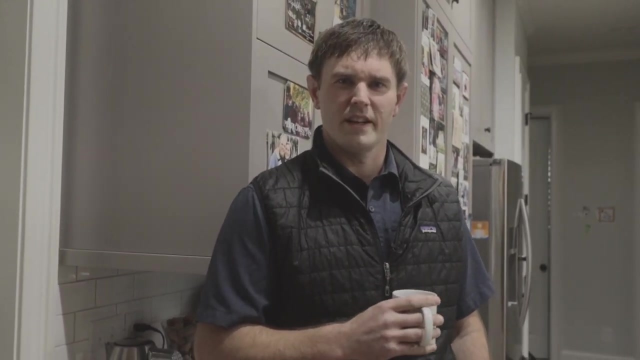 Favorite meal as a kid? Probably my mother's mac and cheese. Every child should answer that question in the same way. actually, What's your favorite healthy snack? You know, I'm kind of on these almond butter cookies, The Nature Valley. 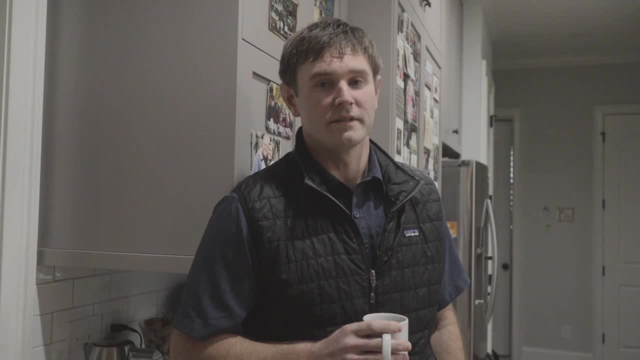 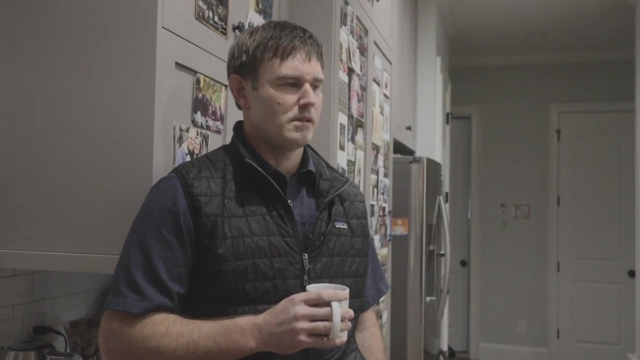 I'm kind of on those kicks right now. They're really good. I'm going to consider that health food. Then what's your favorite guilty snack? or cheat meal? Ooh, You know, I'm just always down for Tex-Mex, like Diablo's. 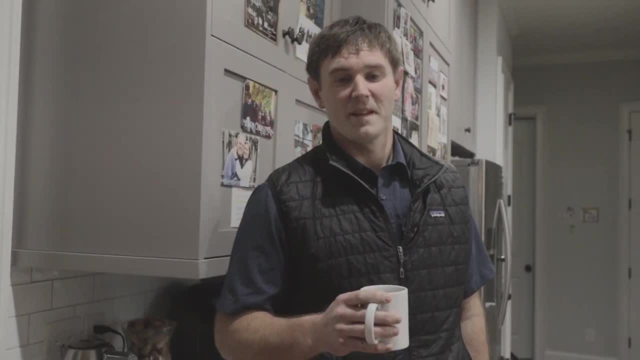 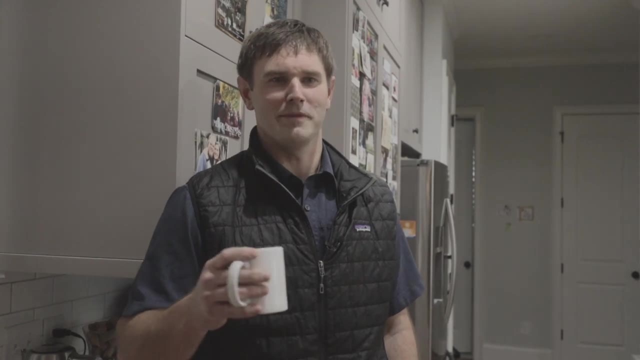 Yeah, Chipotle, stuff like that, Great choice. Yeah, All right. controversial question: Pineapple on pizza, Yes or no? I mean, I think pizza redeems everything. Like you could put anything on pizza so sure. 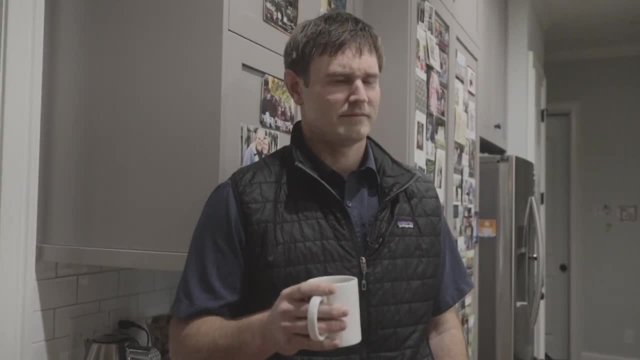 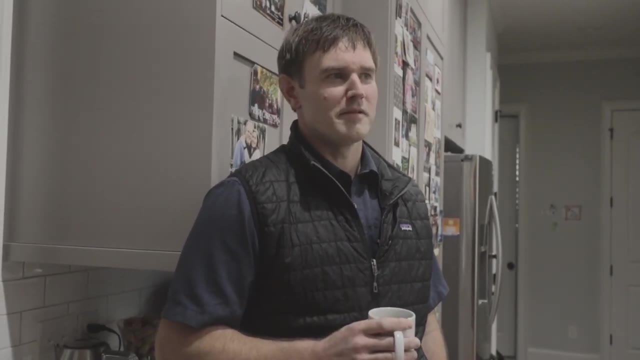 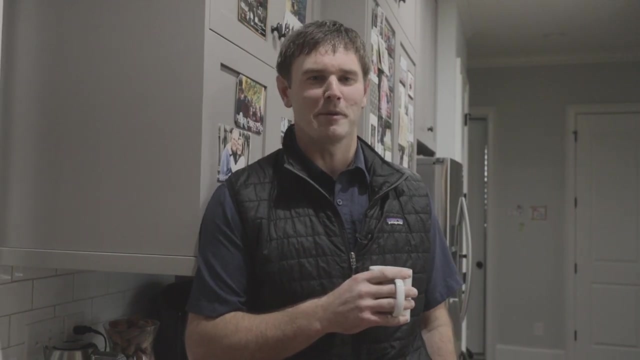 Okay, Apple or Android Apple, It just works. Any artistic hobbies you keep up with. I've always been a musician, so I like to dabble a little bit and play on the piano and try to play some of the Hammer Dulcimer sometimes. 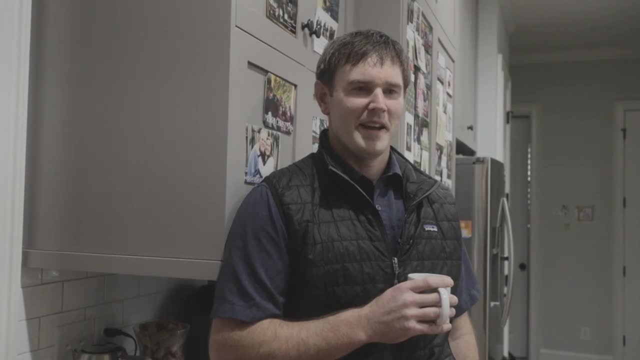 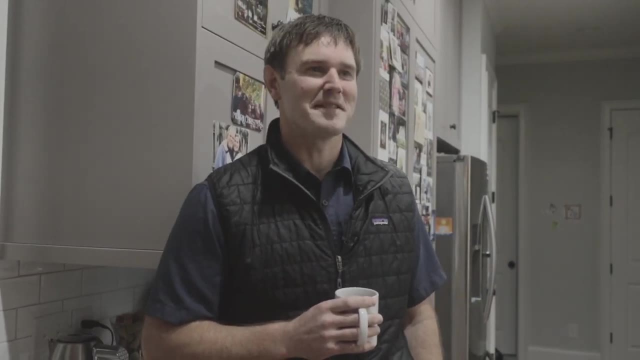 What kind of music do you listen to in the clinic, Man? it's kind of a mix. My son's got me on a lot of movie soundtracks now, a lot of Christopher Nolan movie soundtracks, Hans Zimmer and stuff like that- these epic movies. 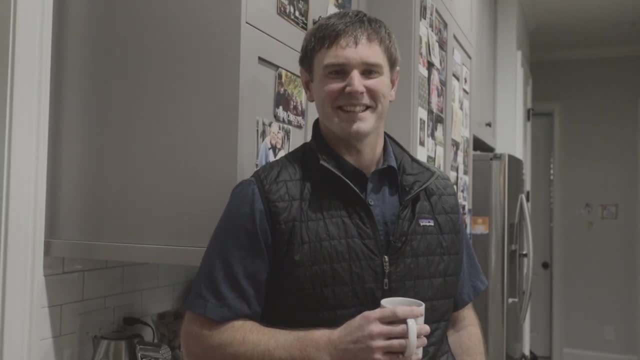 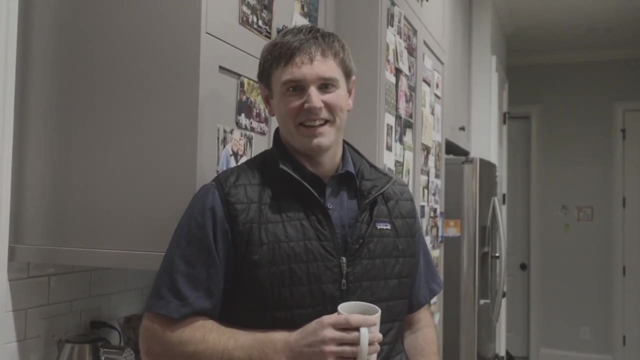 My clinic. my staff just kind of makes fun of me when they hear the epic movie music. Do you ever have to put on stuff like Kidz Bop or anything like that to calm your younger audience down? You know my kids love to listen to Kidz Bop in the car. 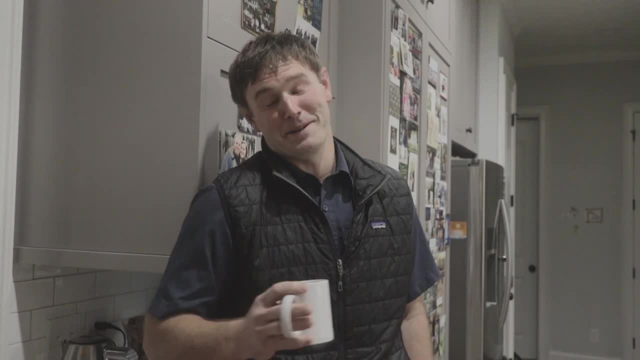 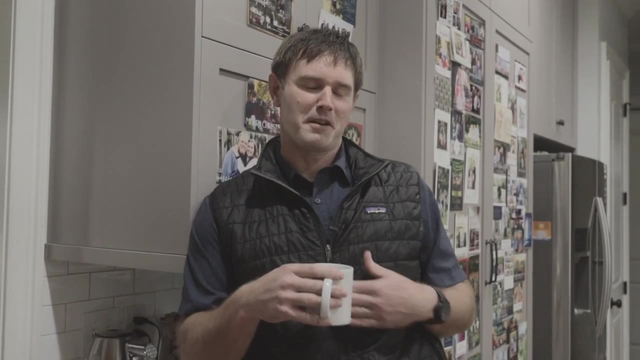 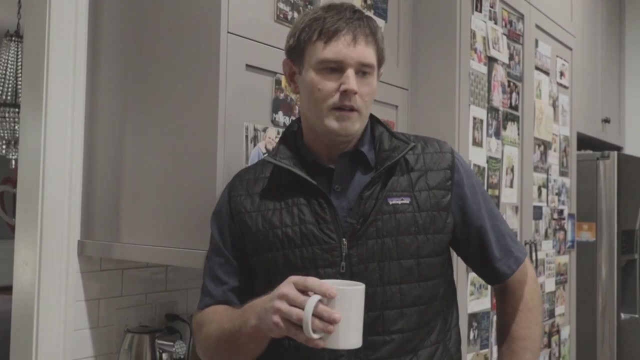 I'm not a big fan of Kidz Bop, so I try to put it on something else. That's just been my selfish part of me. of course, What's the best way that you relax after a long day? You know, I think, just sitting by a fire with my wife and getting to catch up. 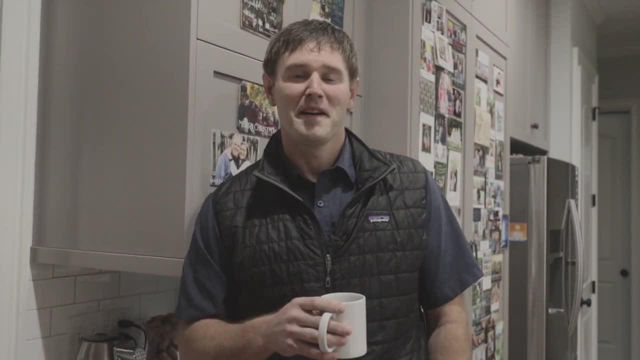 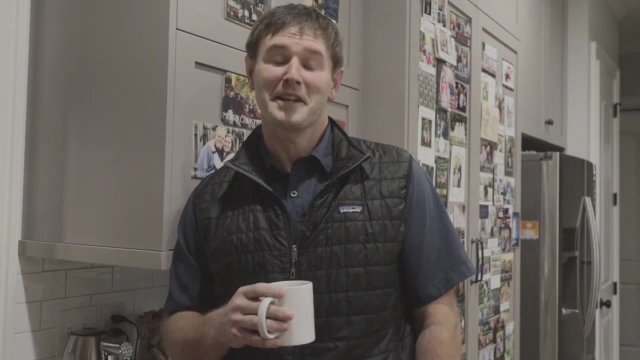 Oftentimes we don't get enough time to do that, so that's one of my favorite things. Most of the time, though, if I'm sitting down and it's a long day and we get the kids in bed, I'm probably going to fall asleep on the couch in pretty short order. 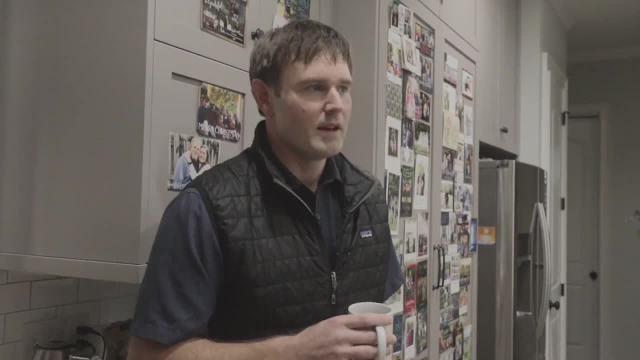 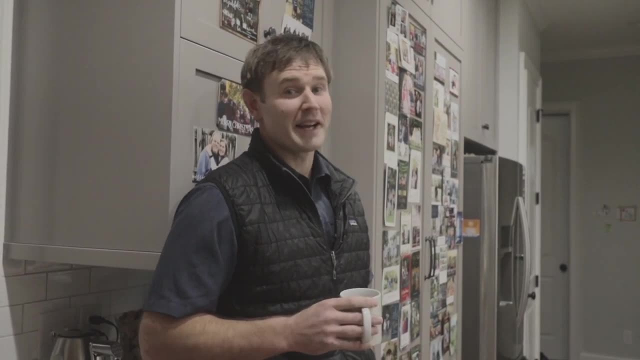 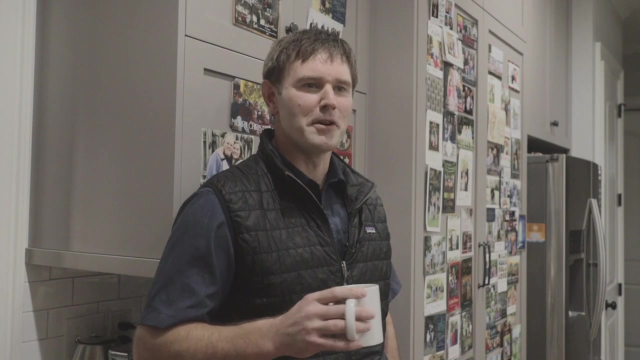 Night in or go out on the town kind of person. You know I'm probably more of a get out and do something kind of guy. I'm not sure on the town is the right, but I like to go to shows or take my wife on a date or do stuff. 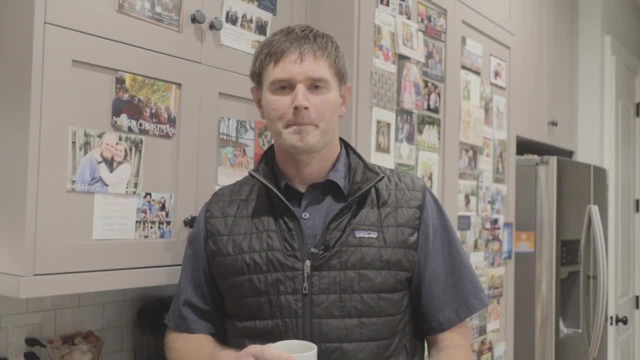 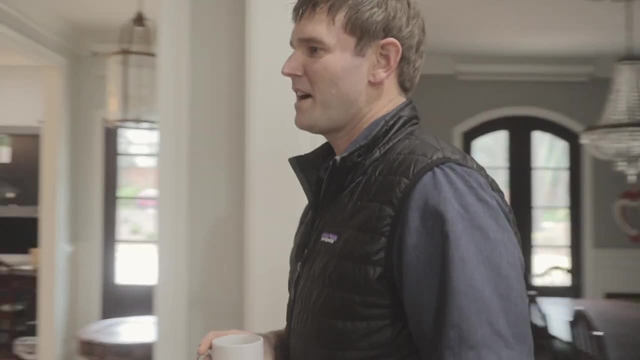 I kind of balance her. She's more of the homebody, Indoors or outdoors person. Definitely outdoors, Yeah, without a question. Beach or mountains, Mountains- I'm totally a mountain person. The beach is nice but nothing beats the mountains. 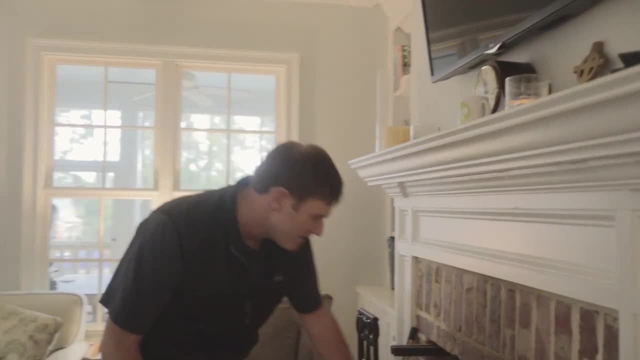 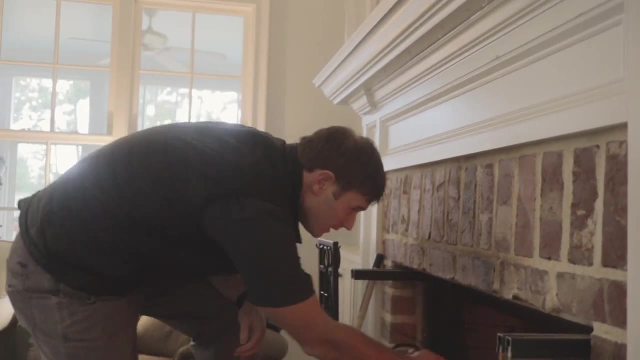 And would you consider yourself more of an introvert or extrovert? I'm definitely more of the extrovert. I always felt like I come alive a little more when I'm around people. Was that personality trait a factor in you choosing your spouse? 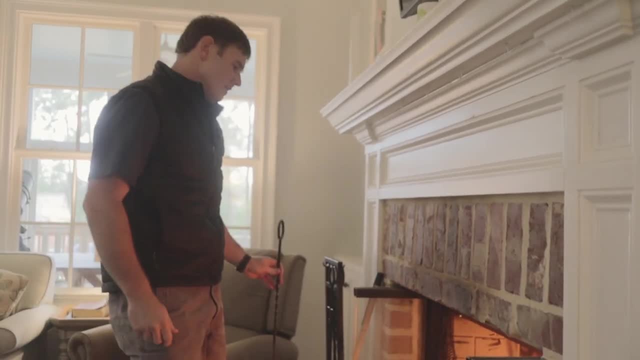 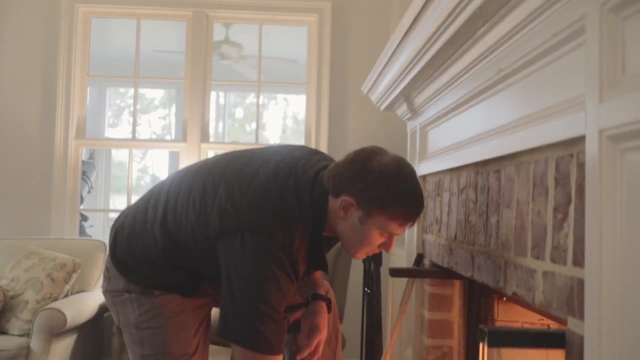 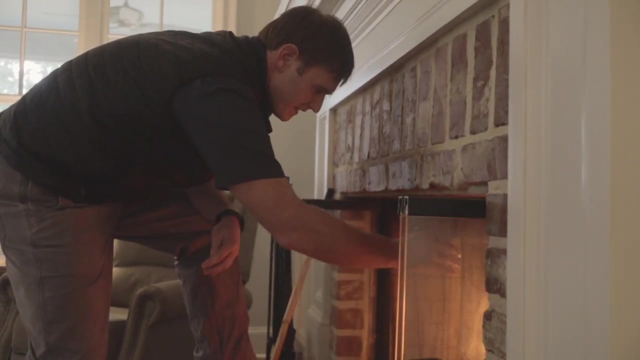 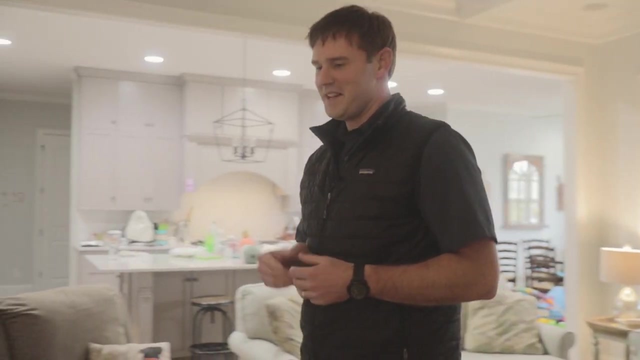 Specialty? Probably. yeah, I mean I think when I was in medical school I was around. it wasn't until I was in my pediatric rotation that I really felt like I was just coming alive, just being around kids, interacting with them, getting down their level. 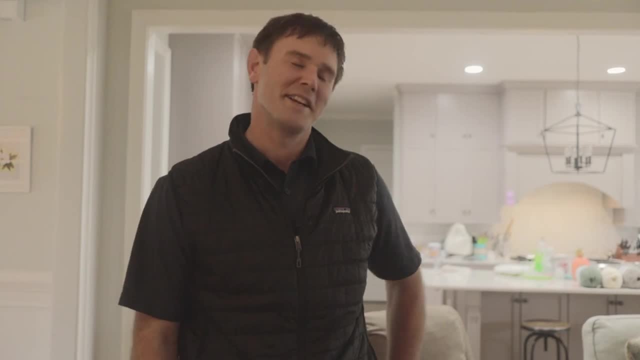 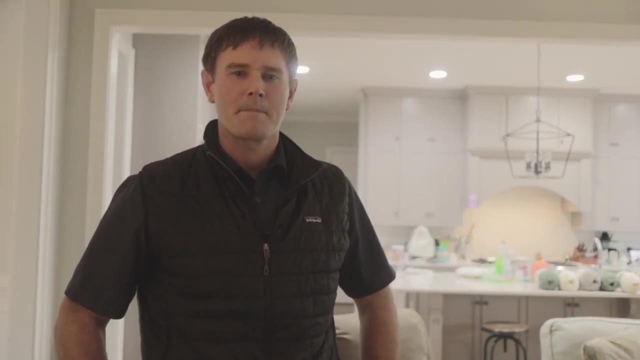 just being a little bit of a ham. So that's kind of my outgoing personality, I guess. All right, so thank you so much for your time. As we wrap up, I want to ask a few more reflective questions. All right, You want to sit down? 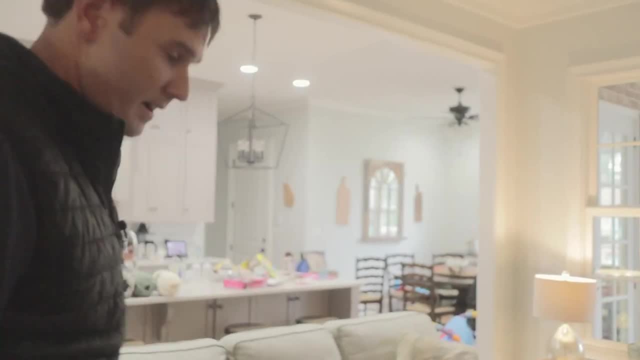 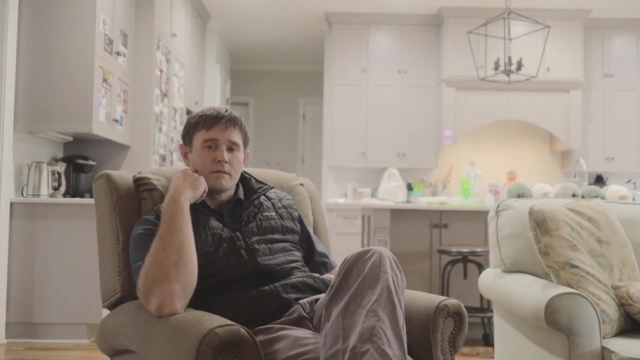 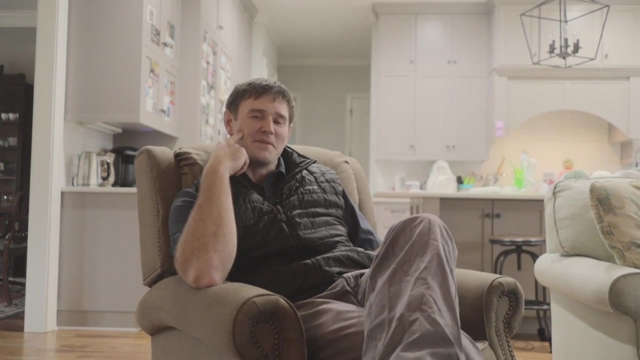 Sure, Yeah, You can sit here. Can I do this across? Yeah, Perfect, Perfect. So what did you think you were going to be when you grew up as a kid? I was kind of a nerdy kid, And my cousin, who was like 10 years old, 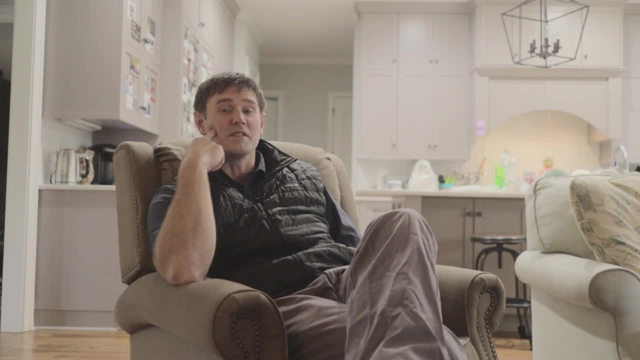 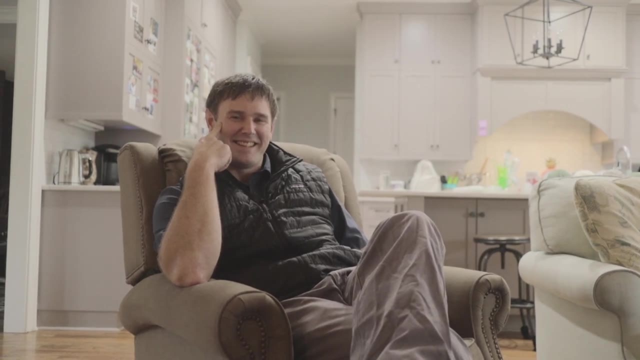 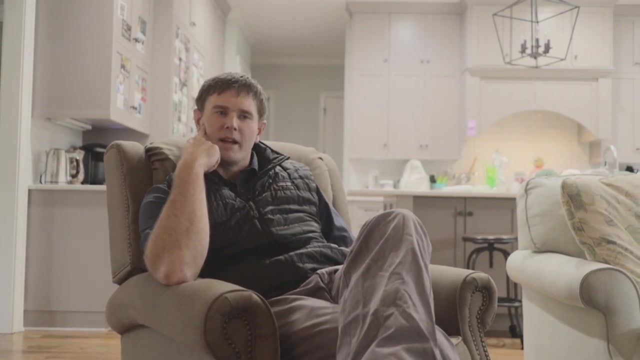 older than me. she was an accountant, So I thought that was awesome. So I always thought I'd be an accountant. I didn't know what that meant. Is there a different specialty you think you could have done? Yeah, I mean, I would have loved family medicine absolutely. 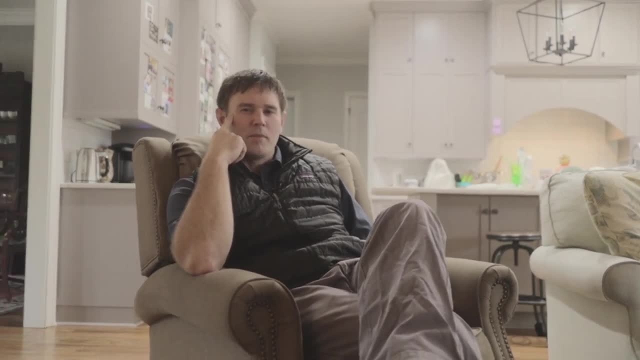 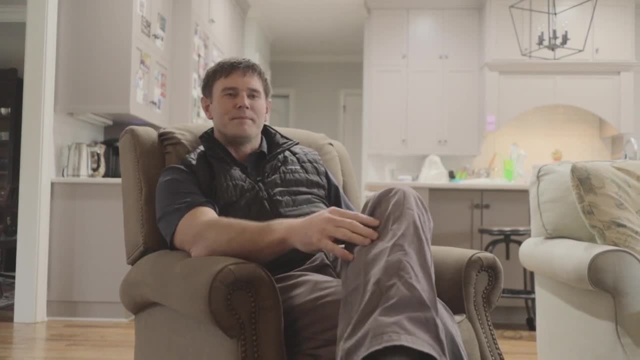 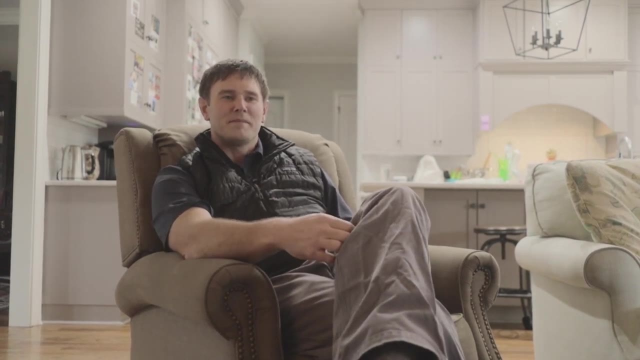 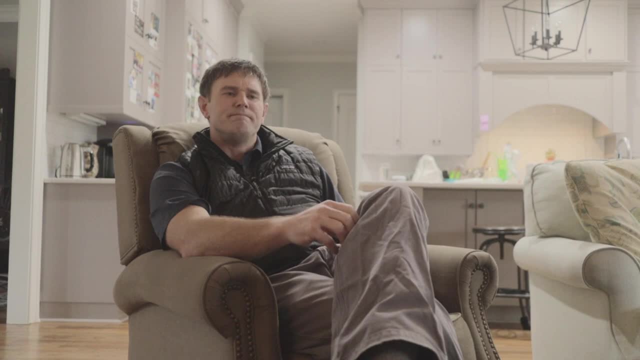 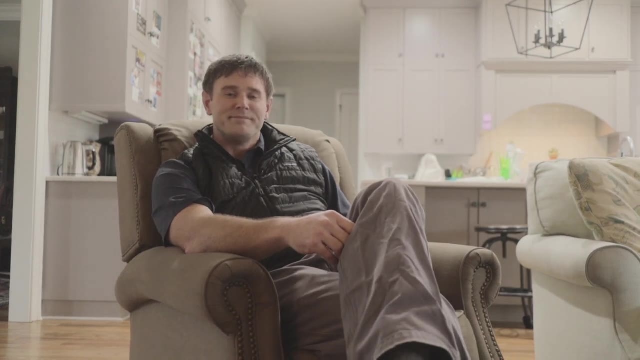 if that's not so bold to say So. I think primary care is definitely. I could have been happy in a lot of those specialties. So if you didn't do medicine, what do you think you'd be doing right now? Hmm, Hmm. 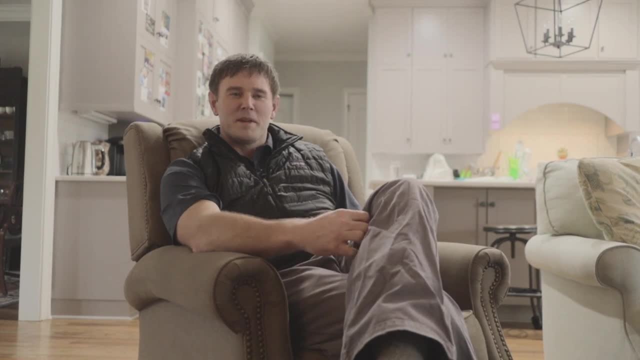 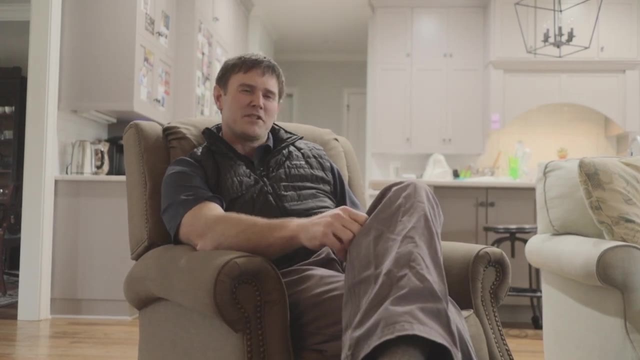 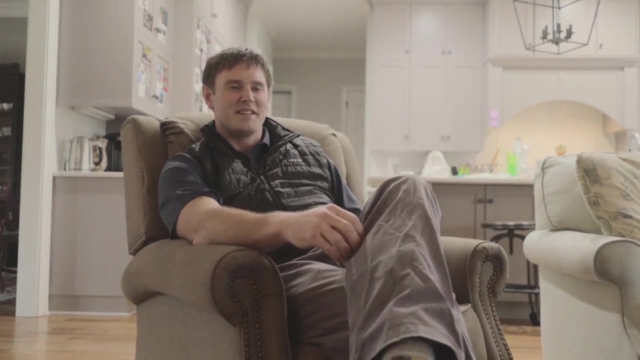 I don't know. I always said if I wasn't a people doctor I'd be a good car doctor, Maybe an auto mechanic, I don't know. I also like carpentry. Carpentry has always intrigued me, Just working with my hands, which seems kind of weird because I just talked about being 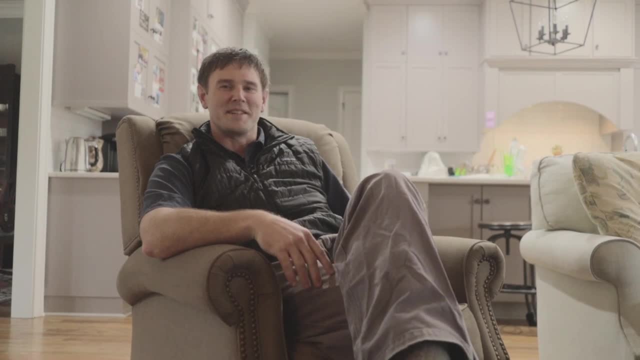 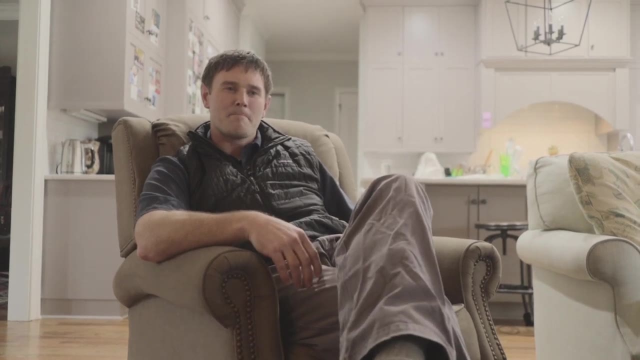 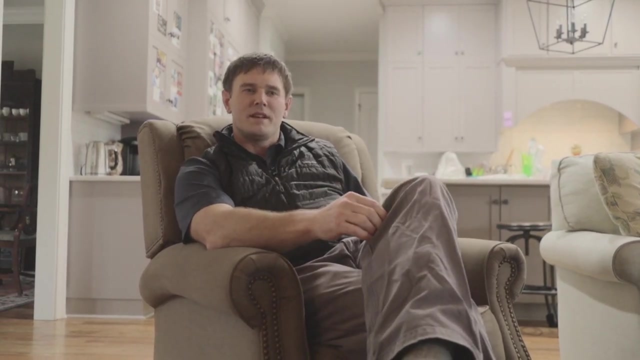 relational, but doing stuff like that has always intrigued me. I'd love to be better at carpentry and stuff like that Were there any times you doubted you would make it as a doctor. No, I mean, I just kind of felt I mean it was hard. Medical school was hard along the way. 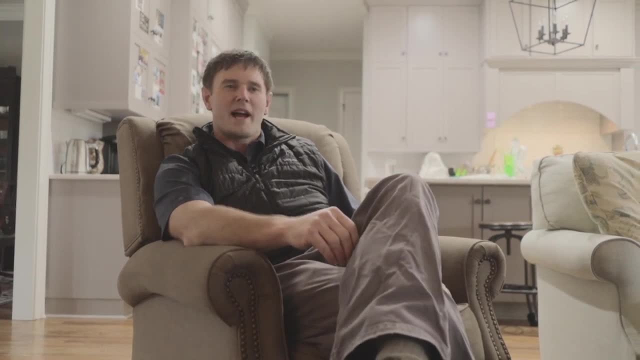 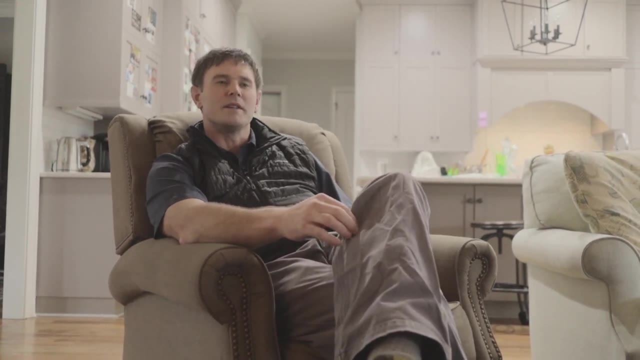 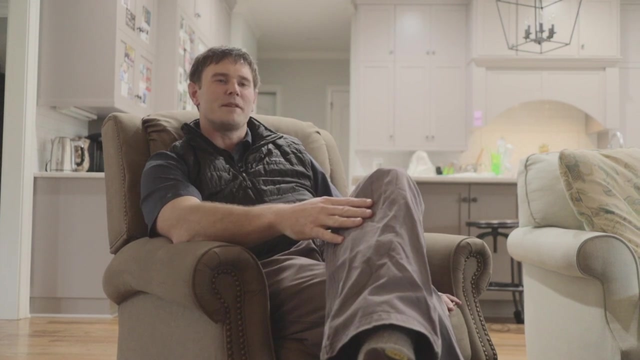 Certainly, there were places that were super challenging, discouraging, especially when you're in the wards and you're working long hours. You know, I just always knew that this was God's design, This was this place where I was meant to be, and so I just always took the next step. and here we are. 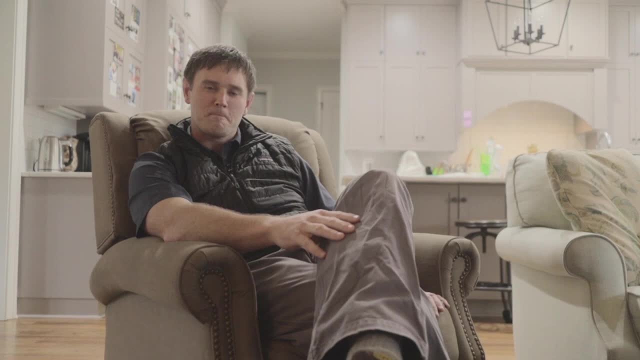 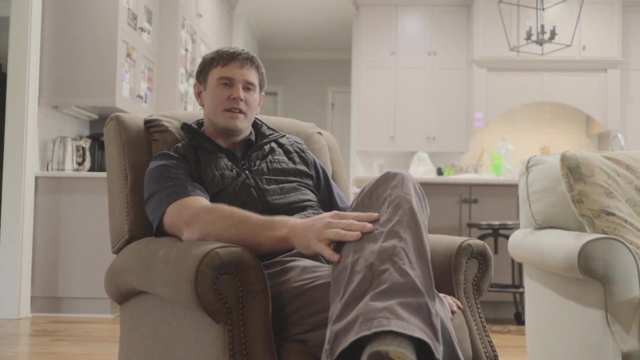 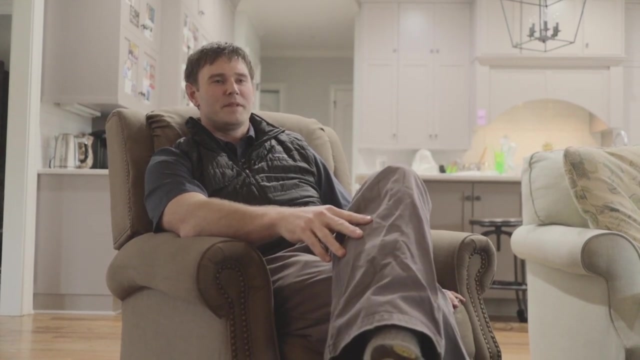 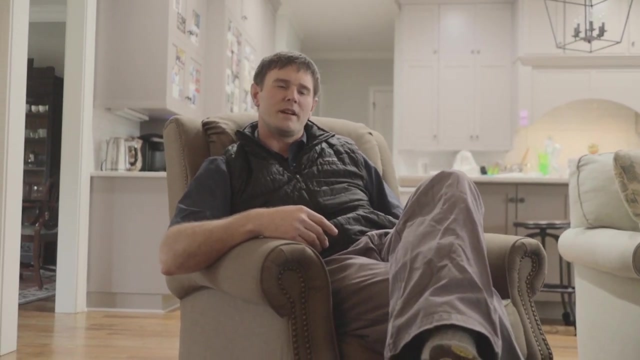 If you could change one thing about the medical field right now, what would it be? I think I would. If I had the power to change it. I think the whole, the whole payer systems I would change. You know, certainly I don't think I would change it in a way. 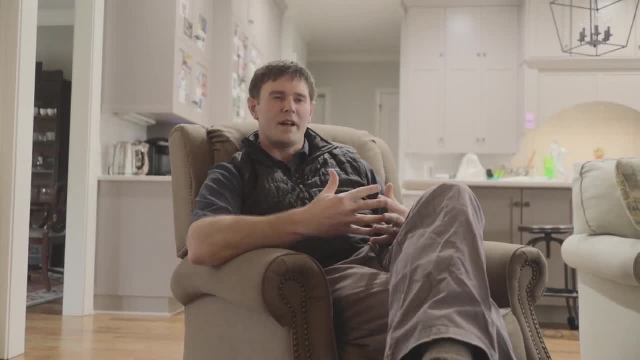 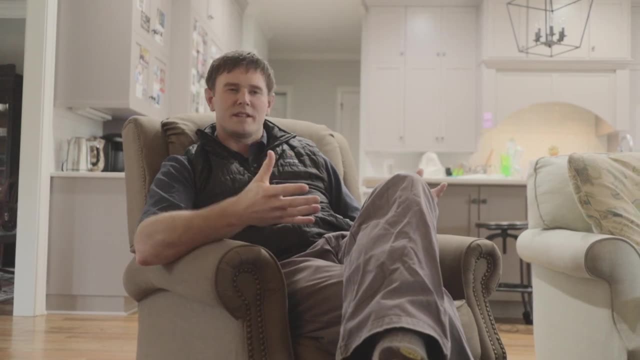 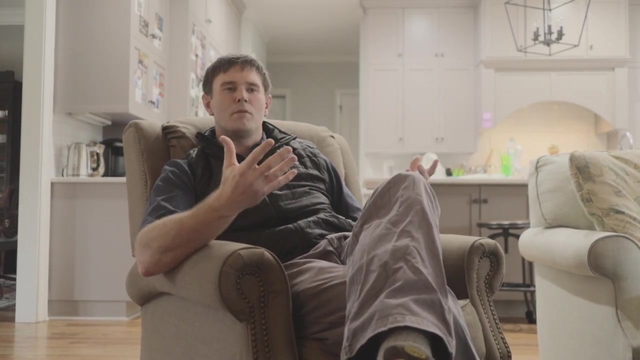 that would make you know there be a one-payer system, but there's a lot of excessive payments for seemingly minor things. I think it's ridiculous that you know for a procedure you get reimbursed for this exorbitant amount of money, while if I spend, you know, an hour counseling an 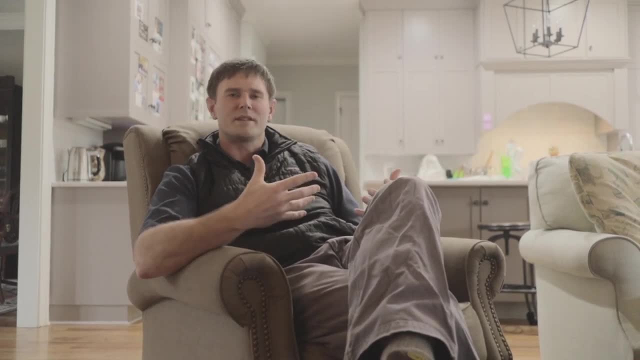 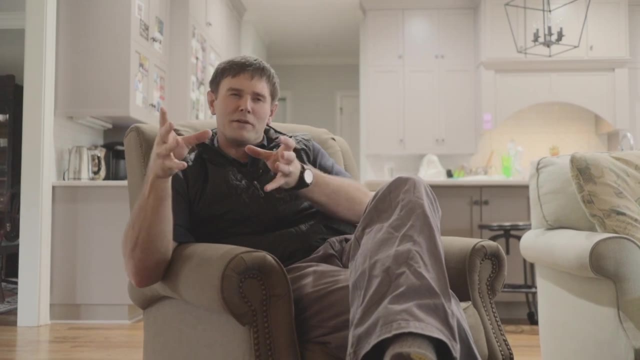 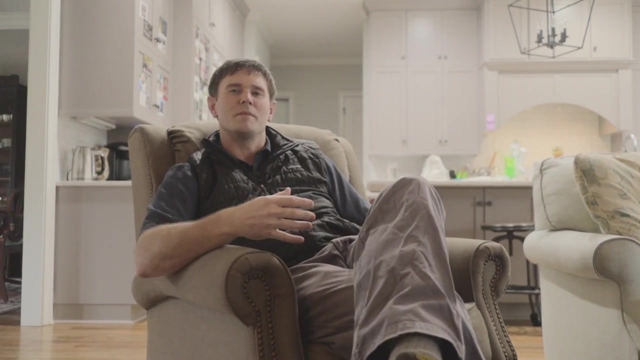 adolescent who's just depressed and even suicidal, like that is. you know the value for it's not so much what you get paid, but it's the. the value is less and I think the value in, in counseling and speaking into people's lives is so much more than if I'm just, you know, suturing up a, you know a cut. 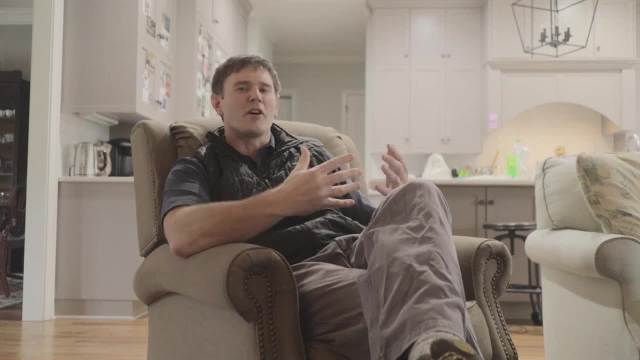 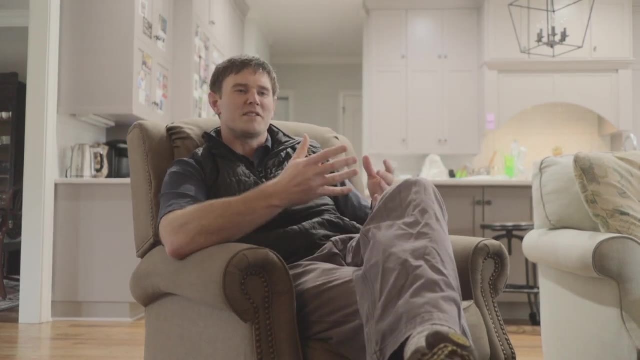 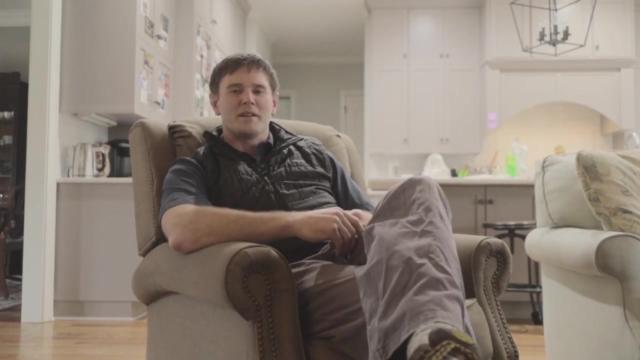 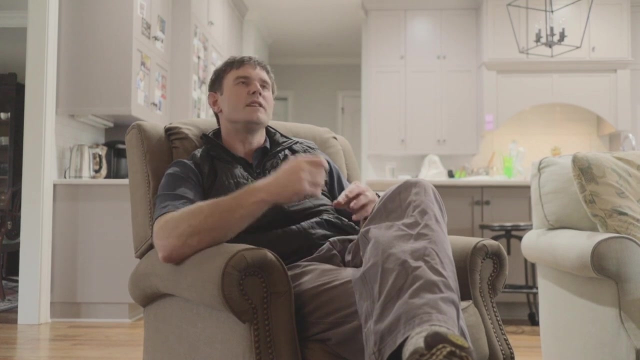 knee. you know there's value in all in all of the healing arts, you know, and so I don't think I don't want to undervalue anything, but I think they're just intuitively there's a value on procedures and I think that those who are working through hard, relational illnesses, associated illness, 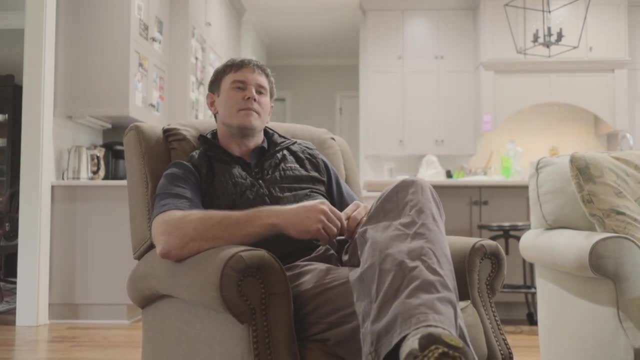 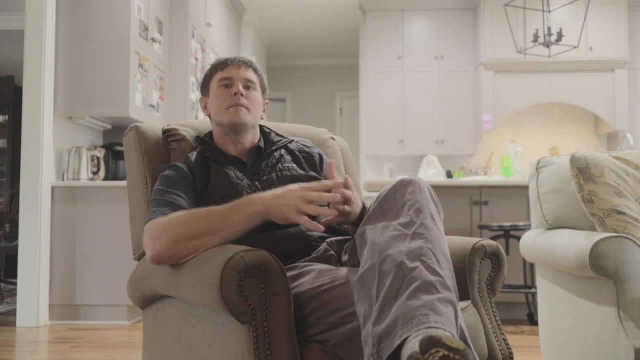 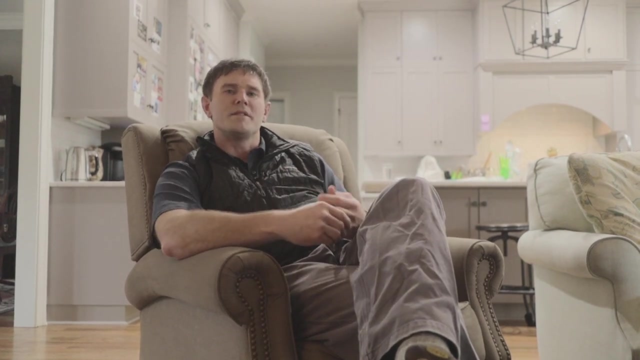 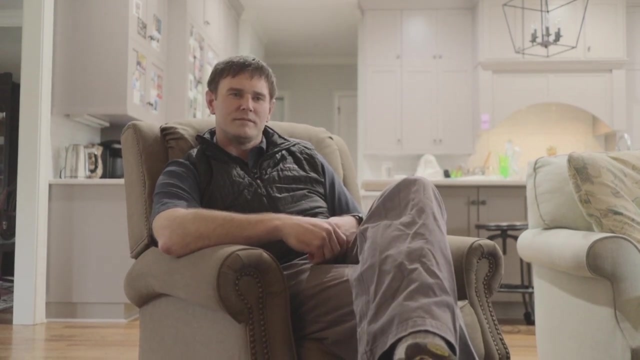 associated mental illness. what am I trying to say this? this kind of time-consuming process that it takes to walk with people through life hardships. there's less of a value for that, and so I'd find a way to make values more equal. great answer. what can a medical student do right now to prepare to go into this specialty? 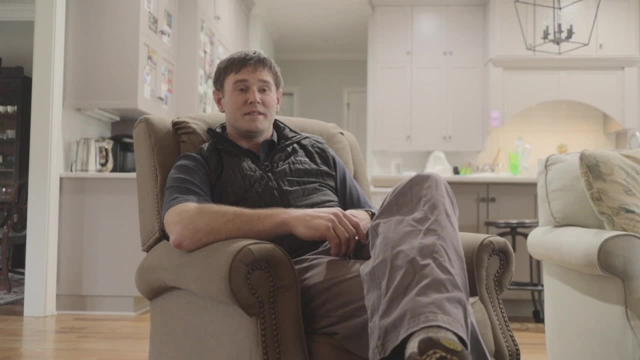 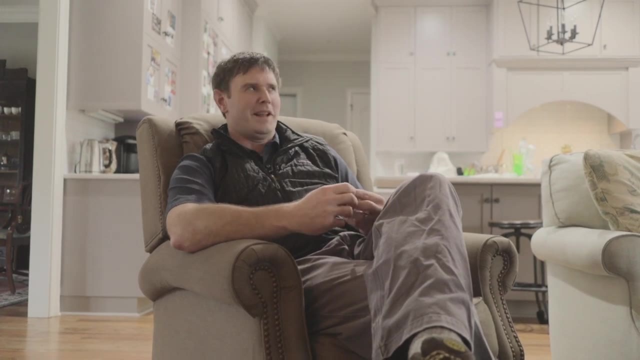 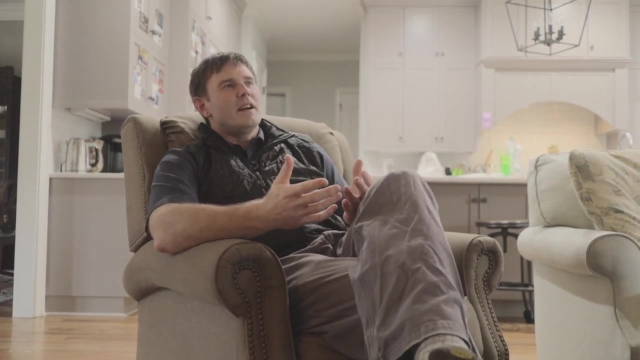 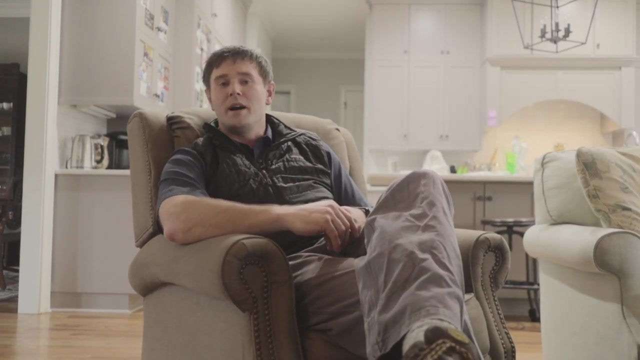 you know, I think trying to expose yourself to children, children, um, to see if you like them, like them, that sounds awful. yeah, uh, you know what i mean by that is like. you know, i mean be a camp counselor. you know, um work with youth groups. you work with the boys and girls club, um. you know, volunteer at your local y go and volunteer. 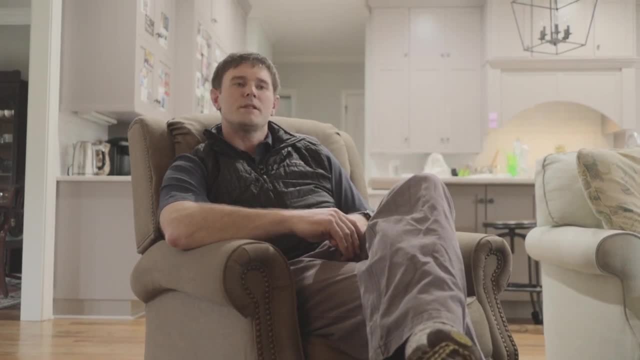 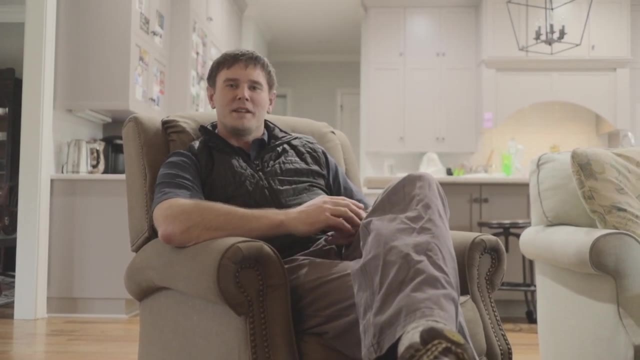 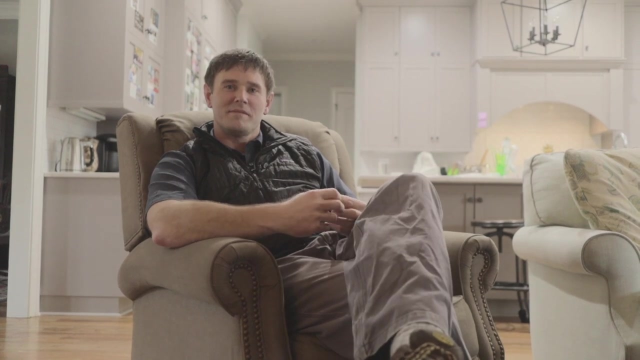 at a pediatric clinic? um, you know, just you know, volunteer in your church nursery. i mean, if you think you want to um help and love children, um, then see if that's something that makes you come alive. great answer. so if you were to go back, would you change any of your experiences? 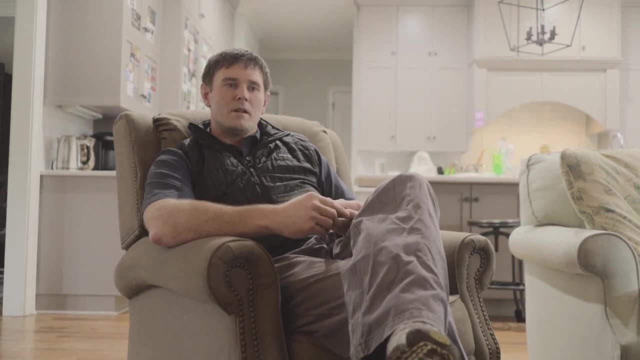 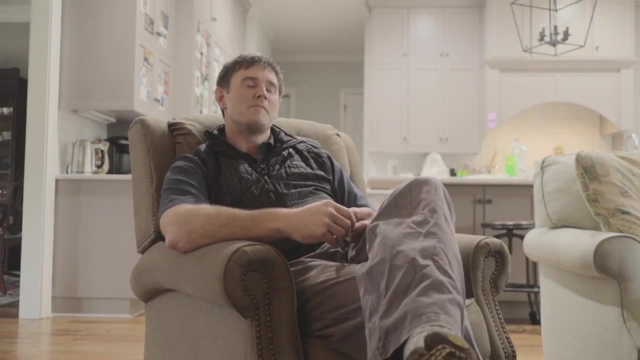 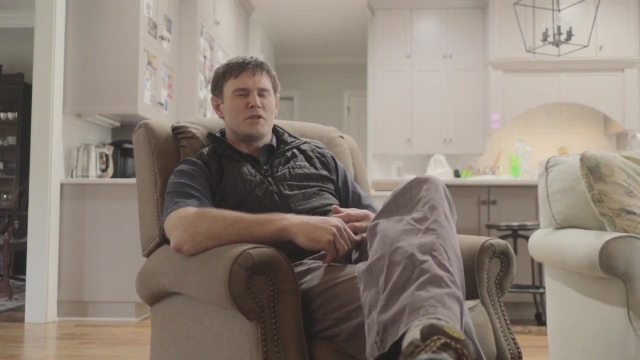 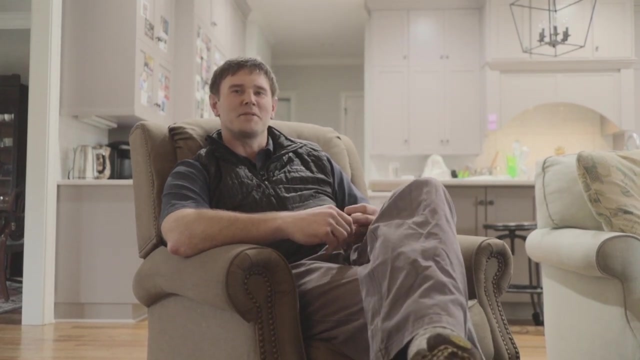 that got you to where you are right now? um, no, no, in fact i've. i tell people all the time, if i people always ask you know, if you would you do medical school again, if, uh, if you had to and i, i would say 100 yes, i would, i would do medical school. that was the time. that's the best. four: 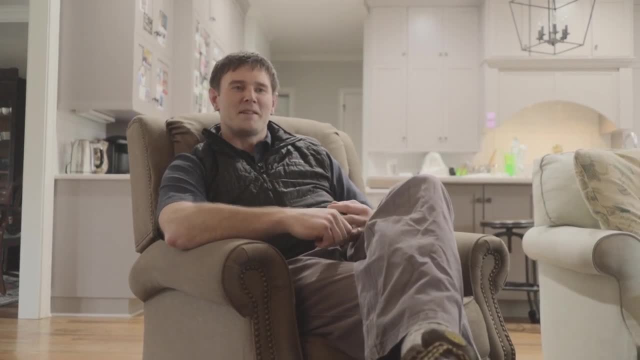 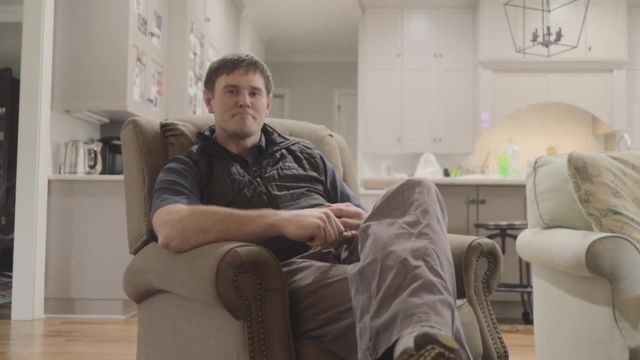 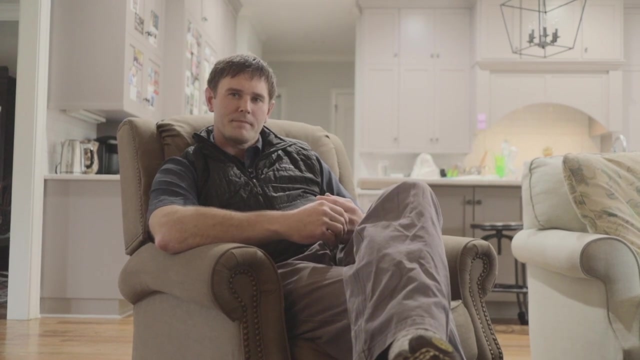 years of my life was in medical school. um and i i wouldn't change anything about it. i loved every moment of it. it's awesome. sounds like i got some stuff to look forward to then. and finally, what would you say to the aspiring pediatric physician right now? 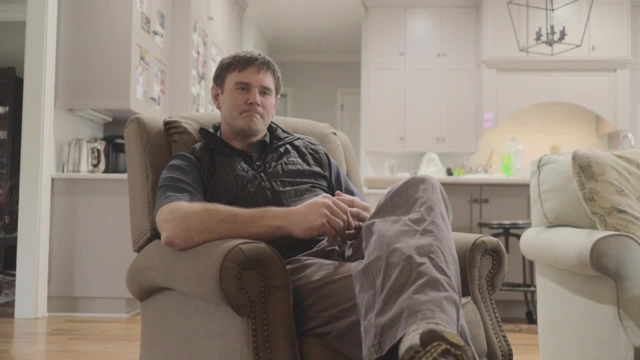 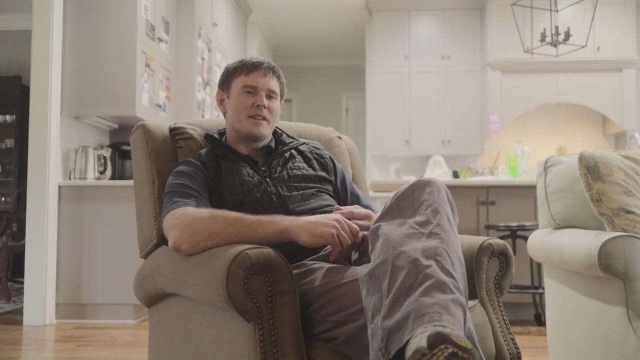 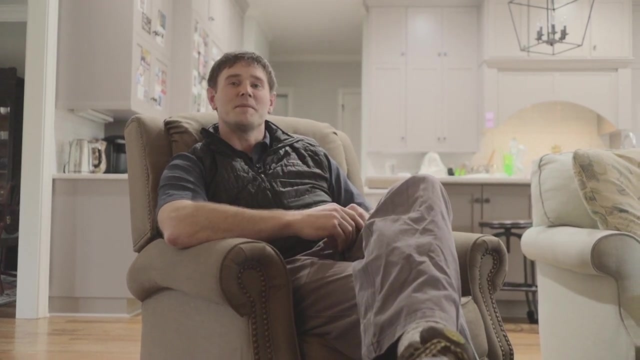 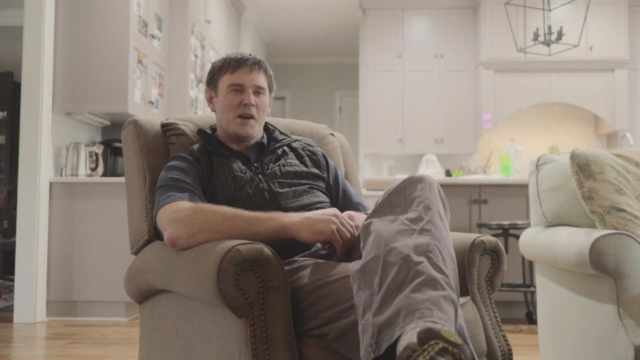 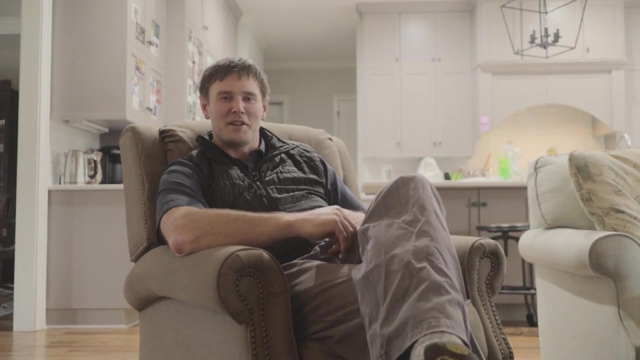 um, i would say, um, sometimes, sometimes it can be a thankless job. um sometimes, um, we, uh, you know, pediatricians are, um, just we're, we're the lowly doctors, or whatever. um, you know, we're not the, the, the upper echelon of of you know who's how much people are getting paid, or whatever. on the pay, 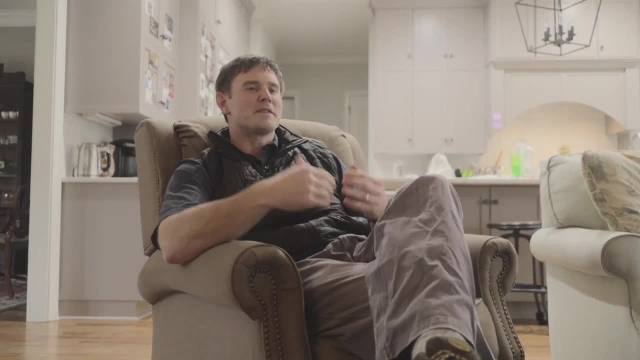 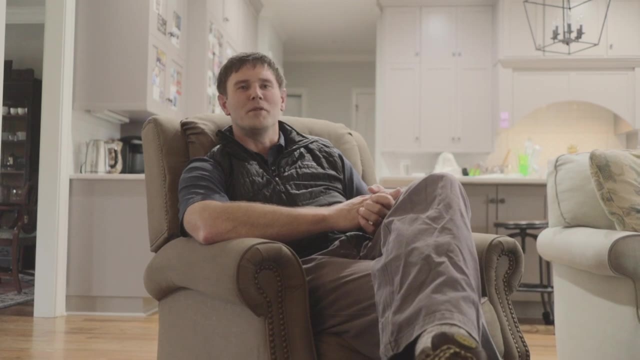 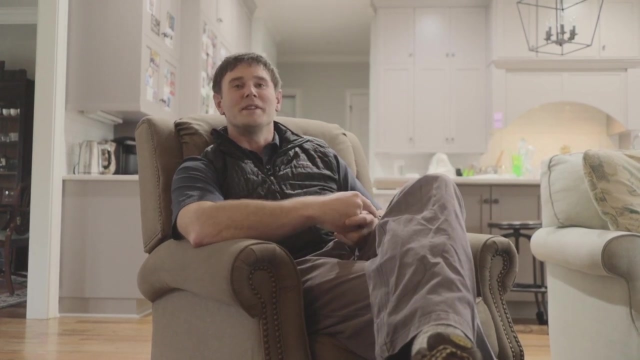 scale, um, but life is about way more than that, um. it's about laying down your lives for others, um, and especially for the vulnerable and the weak. um, you know, and i think you know, children are are the most vulnerable in the week, and our job is to take care of children, um, you know, rich and poor.